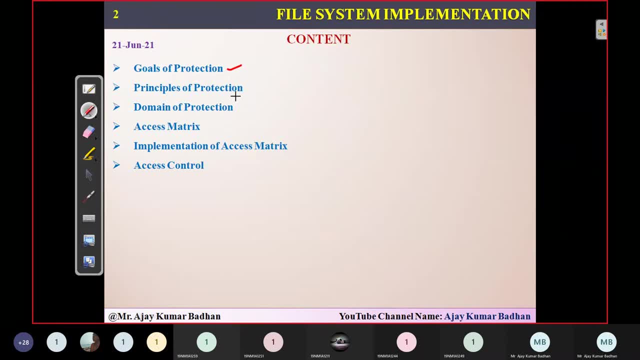 about the goals of protection, what exactly protection is and what are the different goals that we have with respect to this particular protection, and what is the basic principle that has been actually used in order to apply this particular protection. that we have seen it and, apart from that, we have seen about something called as domains. you know domains, Domains are. 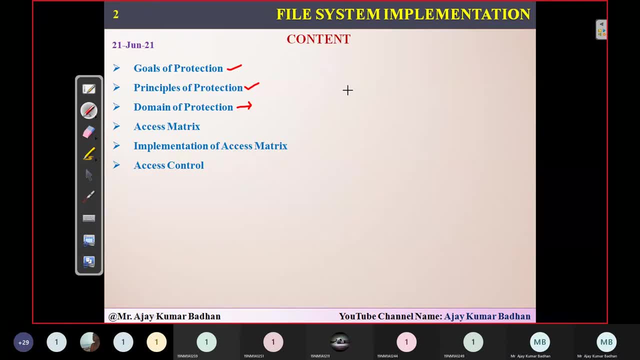 the one where we will be having different, different objects. we will be placing it and using that. objects will be performing operations on that. So what are the objects? what are objects in this we have discussed? objects are nothing but here, something like your resources. whatever the resources we have within the system, we call that as an 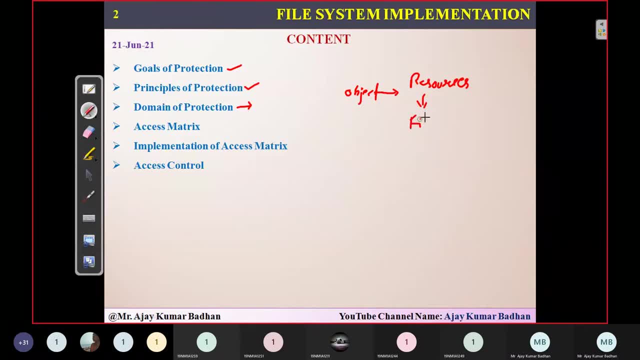 object. So here the resources can be of type, something called as files, or it can be a hardware resource, something like a printer, or we have something called a scanner. So within the system you people might be having files. the files means again: you know that within the files you'll be. 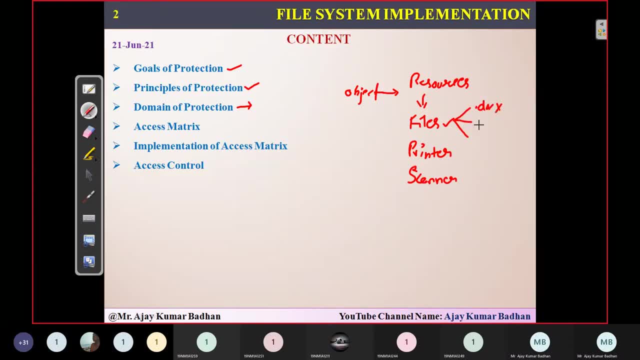 having different, different type of files, like docx files. you'll be having xls files, that is, excel files, document files. you'll be having presentation files, ppt. all these things comes under your files concept. The next thing what we have is this is a hardware- printer and scanner- and I think that the hardware 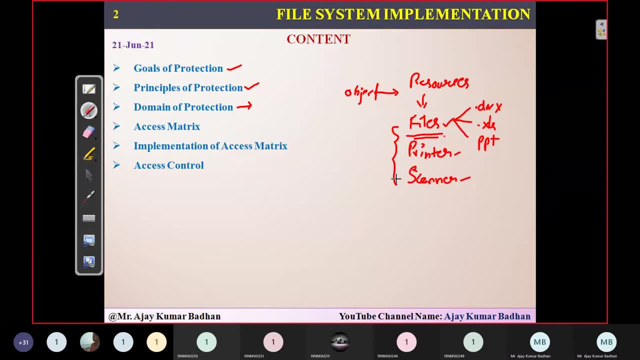 devices which we use. so how to provide protection. so here these resources, based upon the requirements they will be placed with the different, different domains. We also have seen something called as intersection of these particular domains, So this is domain one and domain two, so there might be some. 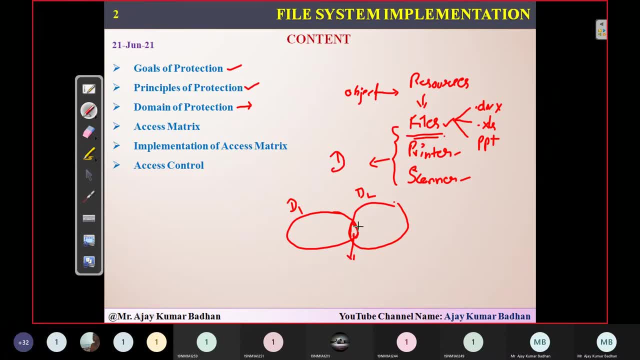 operations here, which will be using it in order to perform different operations here. like you know what we can say, something like a common objects Suppose for all this particular object. this can be used for both the domain 1 and domain 2 and within this we can. 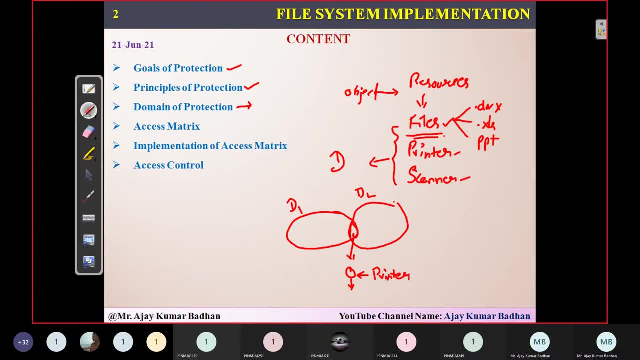 perform the operation. let us suppose print. this is a printer. so what is the operation we can perform on this? that is print. so any process, any process, pi, which is actually executing either in domain 1 or either in domain 2, they can perform an operation on this particular object, that is. 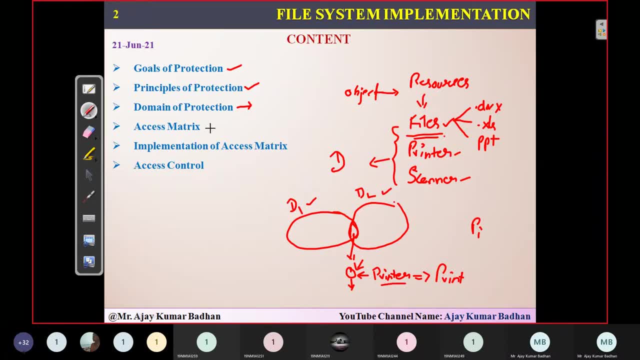 nothing but the printer so they can perform different operations on that. so today we will be discussing about access matrix. so, using access matrix, whatever we have discussed in the previous session, how that can be implemented, how that can be implemented in a format of matrix that we will. 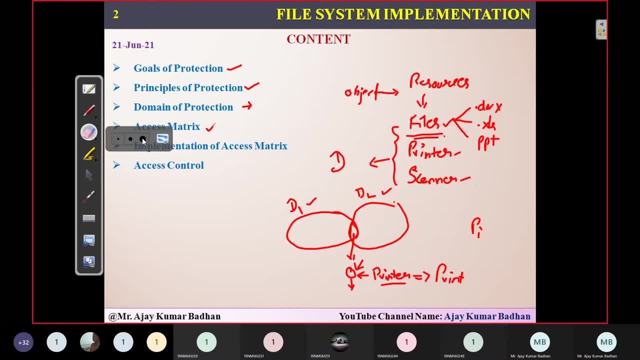 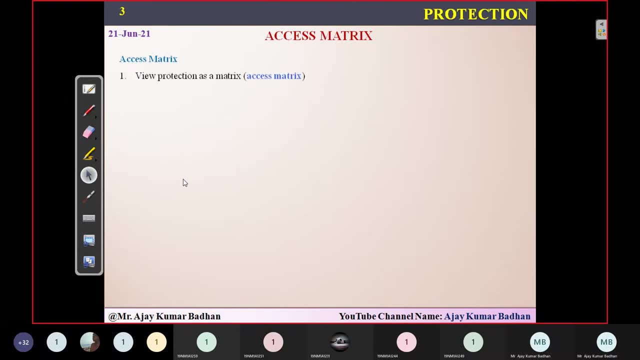 be seeing it in today's session, okay, so let's go ahead so you can see that there is an access matrix here. so what do you mean by access matrix here? nothing, but it is also called as something like a protection matrix. okay, so where we will try to protect, i mean we will be representing. 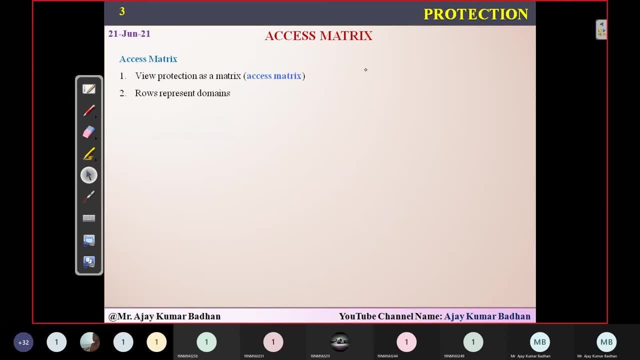 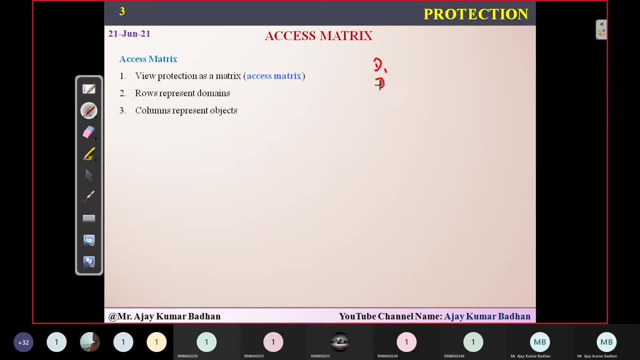 so what are the domains we have? so what are the domains we have? so what are the domains we have? domains are generally represented using something called as d1, d2, d3. each one is one specific domain and within this particular specific domain we will be having objects. i think you people, if 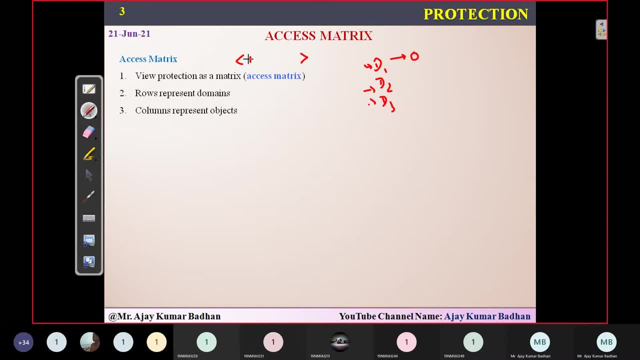 you remember the previous session, we have used a pair where we have represented access rights, isn't it? we have represented access rights, which is nothing, but it's a pair of set where we have d and r. d is nothing but the set of domains, what we have now and on those domains, what are the? 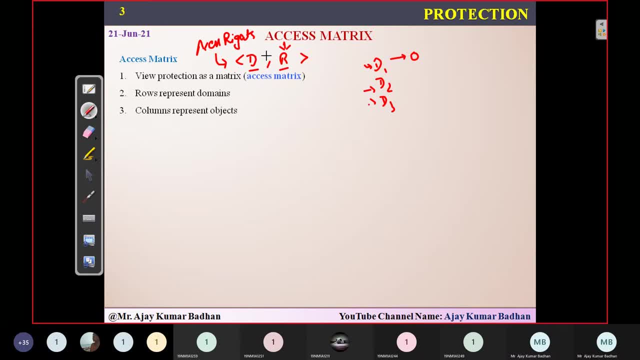 different operations we can do- so that's what we are going to be talking about in this session- can perform. so every domain will have even objects also. we have here objects also here in this particular thing. so what are the different set of objects that are present in this particular domain? 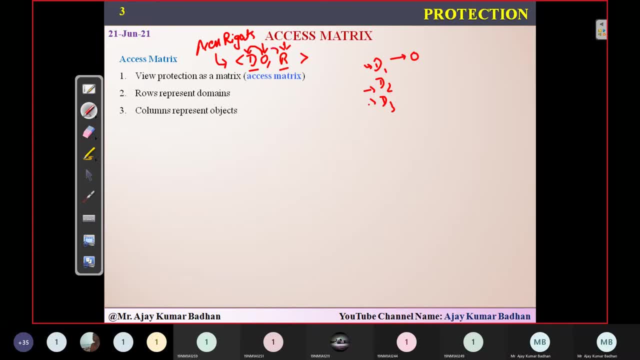 and what are the different operations, set of operations we can perform on that particular object with respect to that particular domain that we have discussed in this particular? so that is what he's talking about here: access matrix here. so here we are going to see how. so here this address access matrix, as you know how the matrices are actually represented here. 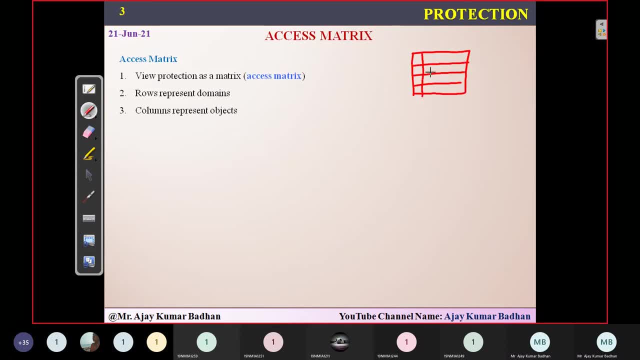 this is a way, right? that is nothing, but it is a set of a combination of rows and columns. so suppose this is 0, 1, 2, 3. this is a row, right? this is a row which we are representing, and here 0, 1, 2. 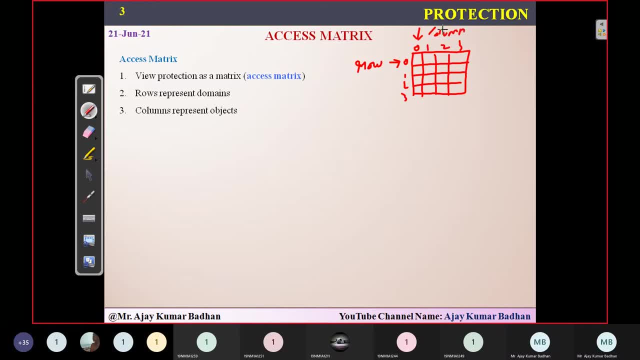 and this is what we basically call it as column. this is basically what we call it as column here. okay, so what is the pair here? 0 comma 0 represents this particular location. so in this way, so we are going to represent our matrix, where the rows will: 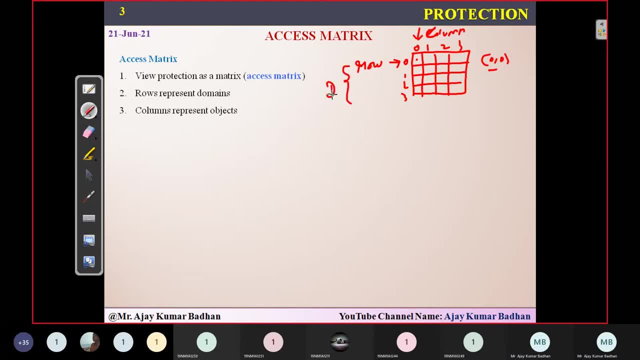 έ represent domain. so all the domains, whatever are there, we are going to represent in a row and whereas coming to the columns, we are going to represent the objects. so, coming to the column, we are going to represent the different objects, what we have now. if you want to access a particular cell in that particular matrix, then you can do it using 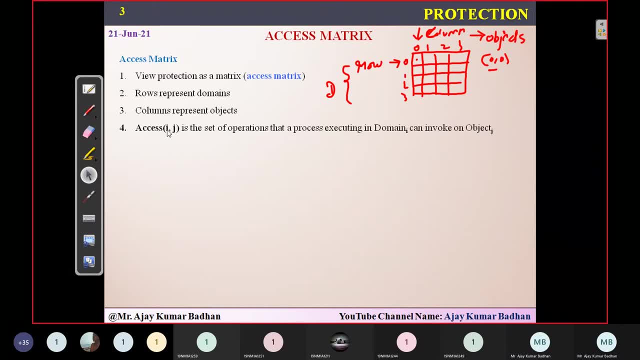 something called as access of i comma j. so i is nothing, but this is the one which is representing the row here. this is the one which is talking about here, so i is represented here and the column is represented using j. so whenever i'm calling it as i comma j, okay, suppose zero comma. 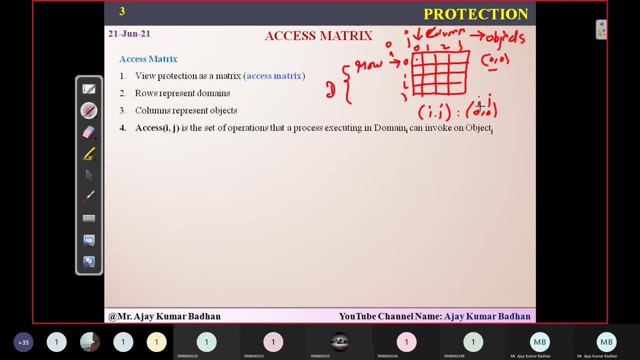 zero. that means zeroth row and zeroth column. so ith row and ith column. so that is this particular column. we are trying to access it. so this is a way how we can use it in order to perform it and the different operations that we can perform on the process. here is nothing but. 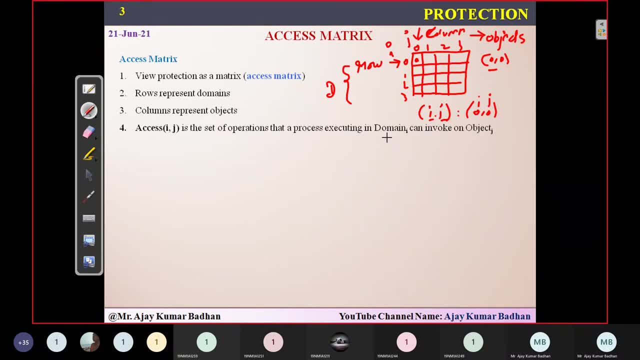 domain i can invoke an object j. what does that mean? here is, whenever you have performing access of i j it means that you are performing some operation on what? on a specific domain i, because i is the one which represents a row, and in the rows only we are representing the domains, so we are performing. 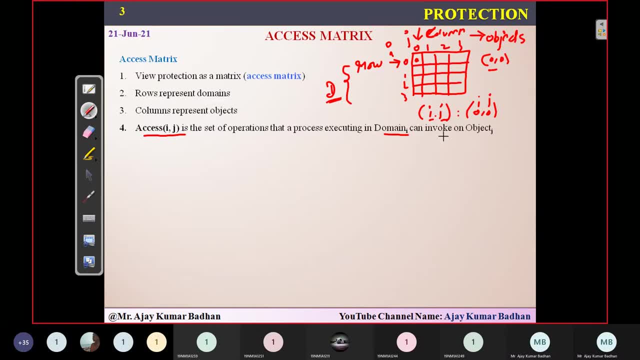 a process is actually executing in a particular domain i by invoking an object, og. so whatever the execution it is performing, whatever the operation it is performing, it is performing on this particular object j, whichever it is okay, represented using a column matrix. so let's see how exactly i will show you the. 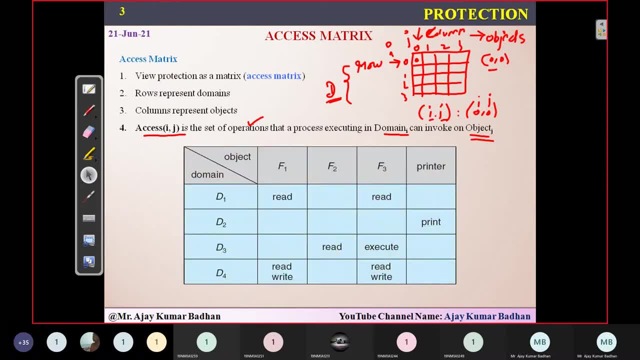 diagrammatic view so that if people can get a clear understanding of this particular thing, so you can see here, as i stated here, the rows, oh sorry, so if you see here in this particular thing, so here this particular row is what i mean. the rows are representing something. 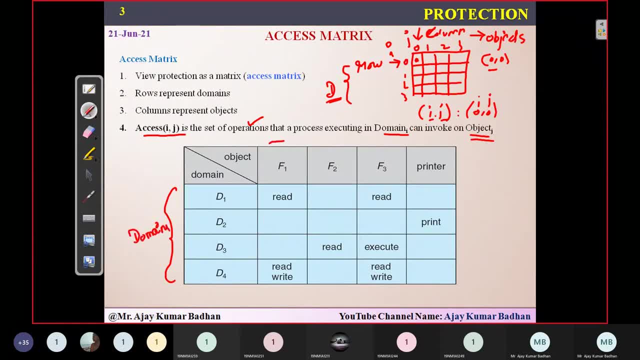 called as domains, and if you see here these particular things, we call it as columns. so okay, this is a row and this is a column. now, if you look at this particular row, so how many? so if you see the rows here, how many? so this is what we are representing here: domains. 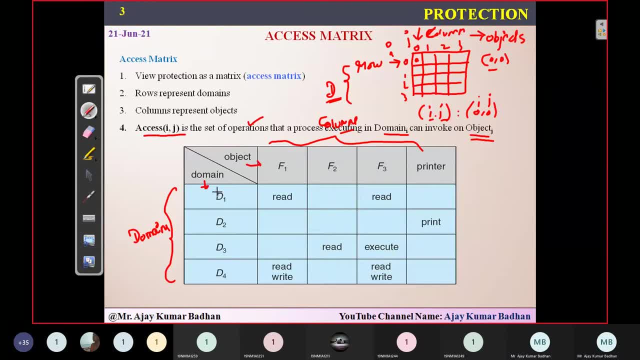 and this is what we are representing as objects here. objects are nothing but, as i stated earlier, these are the resources. so you can see, here there are three, four different type of objects we are having here: f1, f2, f3 and then finally printed. so what do you mean by f1, f2, f3 here? 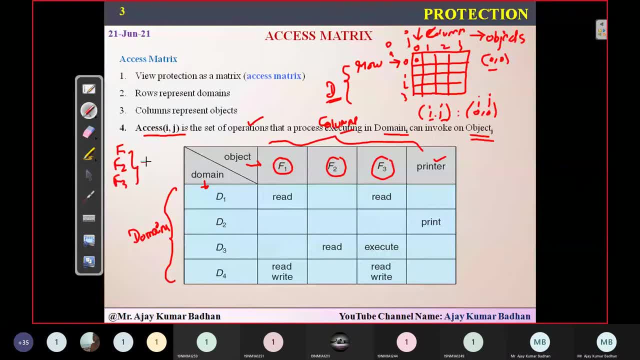 f1, f2, f3. what are these are nothing, but these are the files. okay, so these are the files. the files are represented as this is file one, file two and file three, and this is a hardware resource. what we are having, so objects are nothing but, as i stated, it is a resources. 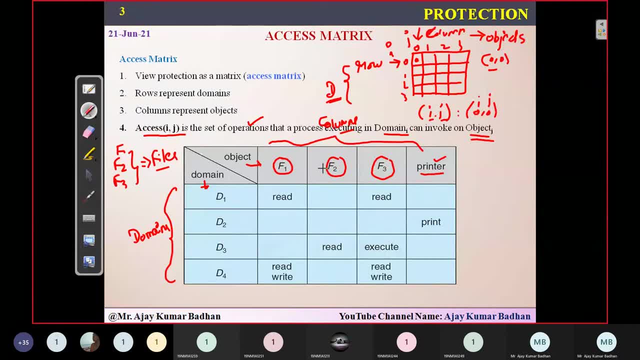 so your printer is nothing, but it is a resource. and file one, file two, so these are the software resources. what we have- file one, file two, file three and printer is the hardware resource and when you talk about this, particular rows. so here we are having four different domains. 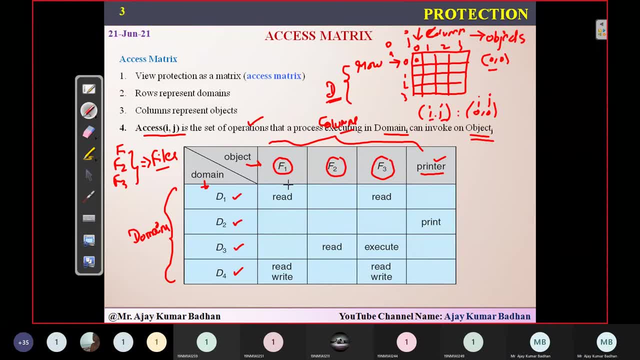 d1, d2, d3 and d4, and whatever the internal cells are, the files are represented as this. you are seeing here this particular cells. these are the ones which actually specify the different operations that we can apply on this particular matrix. okay, so these are nothing but the different set of operations, what we can perform on this particular matrix. 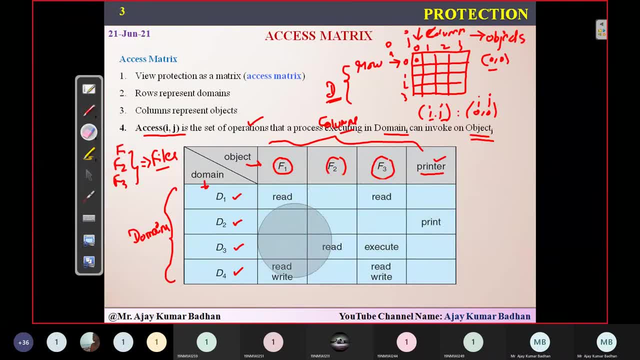 so what are the operations we can perform here? so if you see here clearly, if you talk about domain, if, if a process is executing in a particular domain, so let us suppose there is a process p1 and this particular process is executing in the almighty 계 subway, Ben down space in place open class query here, which is actually. 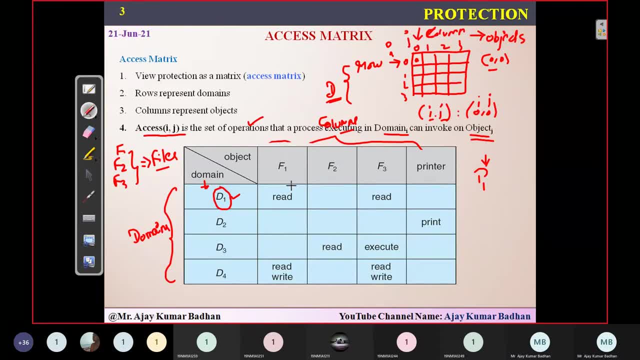 this particular domain, then what are the different? what are the different files that did? but this particular process can access? here is file one and file three and what is the operation it can perform on those particular files is nothing but read operation. so remember, whenever a particular process is executing in this particular domain d1, it can only access only two different files here. 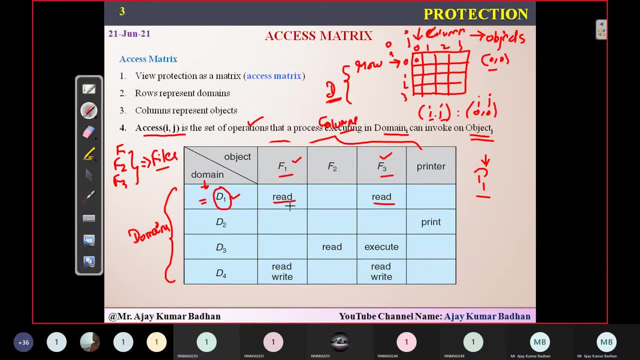 that is file one and file three, and what is the operation it can perform? here is nothing but read operation. it cannot access file number two because there is no operation that is specified here what it can perform, and same way, there is no operation related to the printer. okay, 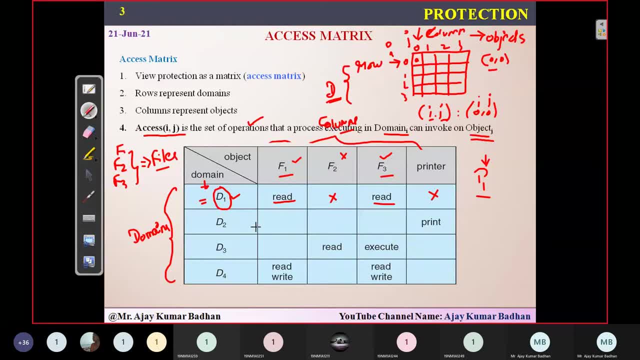 and after this, uh, we have something called as uh, uh, after this, we have something called another domain. we call: okay, it's, if you talk about the second domain d2, what we have in this particular thing. you can see that this particular domain, whenever any process is executing in the 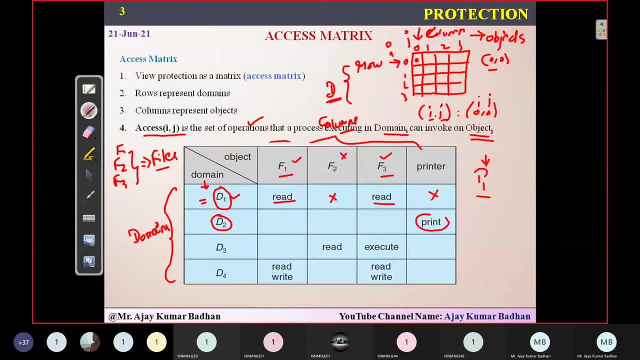 particular domain. it can only access this particular printer. it can perform only one operation, that is print operation. and on what it can perform, here is nothing but the printer operation. the third one: what we have here here, here is nothing but the domain number number three, domain number three here. so if you see this particular domain here, in this particular 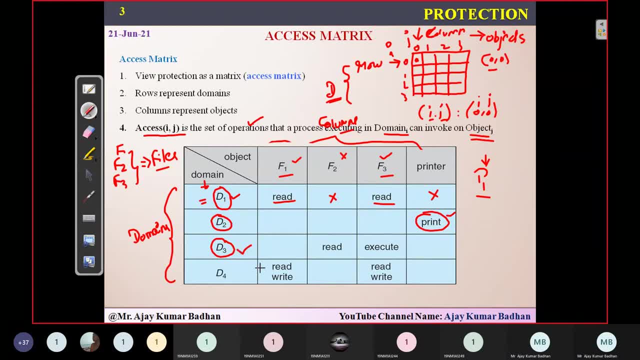 concept this: uh, whatever the process will be executing in this particular domain, it can perform only two different operations. here, that is f2. it can perform operation on file two and file three, and whatever the what are the different operations it can perform? here is something where nothing but. 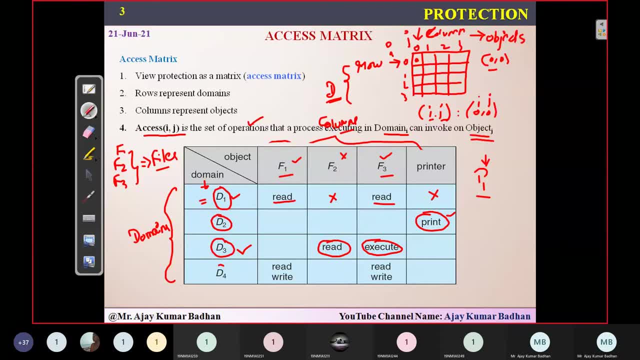 read and execute operations. the third, the last one, if you see, of d4, then d4 you can perform only two different operations means only two different files can be accessed here, something we call it as file one, and another one is file three, similar to your domain one, but only thing is in in this: 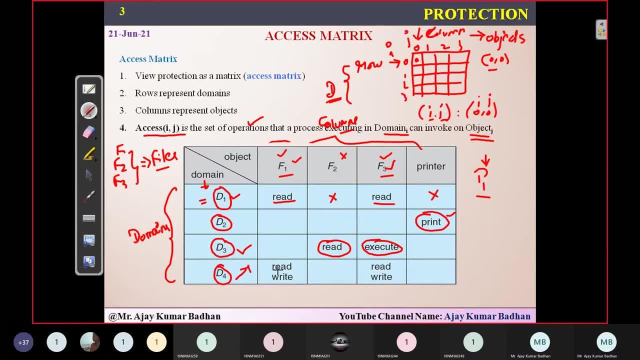 particular case it can perform operation on read as well as write on this particular file. one same way, in the same way for the file three also it can perform the operations. so see here read and write operation. so it can again perform read and write operations on this particular file three. so 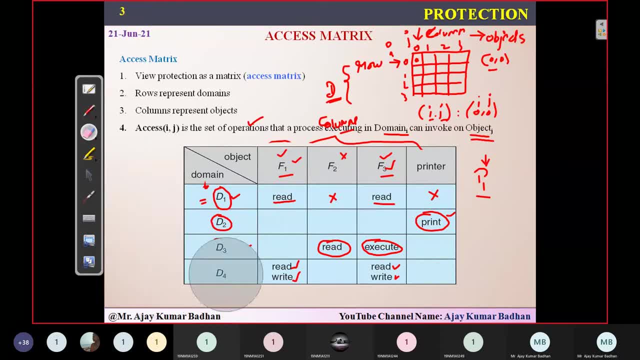 this is the way how this exactly, this particular access matrix, is implemented, where the call rows different domains here and the columns represent the different files, what we are having here. okay, so this is a normal example representation for your access matrix. this is how, hold together, we call it as access matrix. okay, this is hold together, we call it as asus matrix. 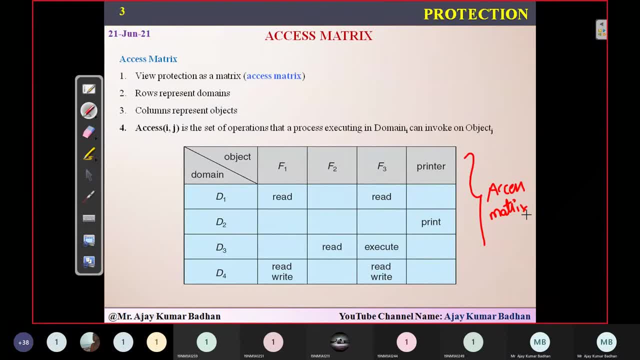 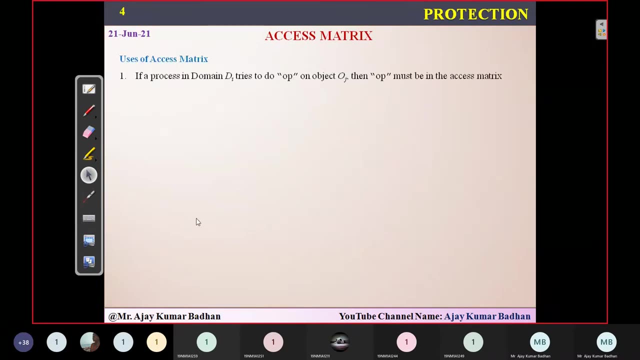 so this is hold together. we call it as a access matrix. so so, without wasting time, let's go ahead. we we need to discuss some different points with respect to this. so what are the use of access matrix here is? so this is nothing, but whatever i have explained. 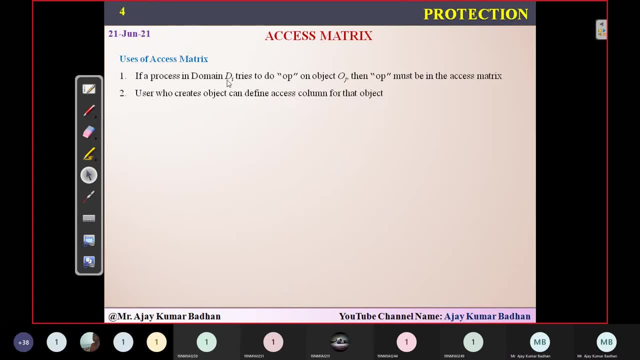 you here. that is what is saying. so if a process in the domain is trying, if a process- you remember a process is the one which will be executing it. so whenever a process is executing in a particular domain, it it will be trying to perform an operation. so what are the different? okay, let me show you the 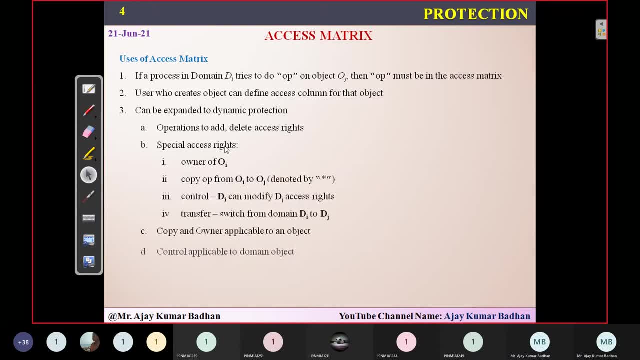 content here and then i'll explain it. if you see here, if a process in the domain is executing, so if di is nothing but any one of the domain di, so i is nothing. but if you take the previous matrix, i mean asus matrix. 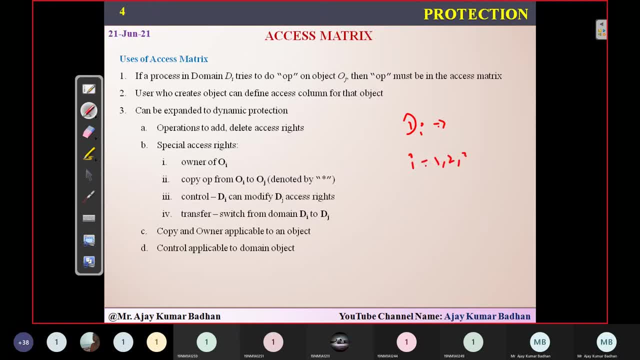 i is nothing but one, two, three and four. so here we will be performing different operation. right, a process may be executing different operation, and that is what is represented using opie. so what are the different operations we can perform by a process on a particular domain? is this? so what is in the texture? 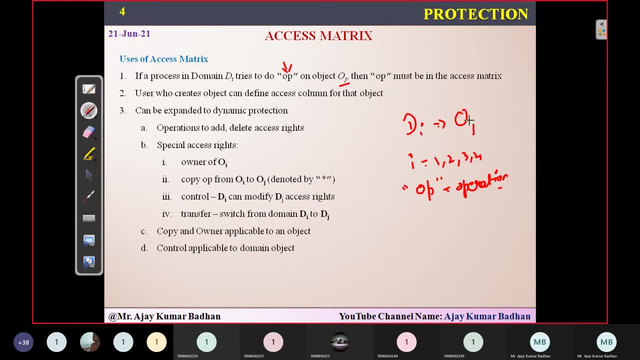 object oj. so oj is nothing, but again oj. so j is nothing but one, two, three, so on how many objects we are specifying here. so in the previous access matrix we have represented how many, four right for f1, f2, f3, and then the last one is something we call it as printer. so these are the matrices. 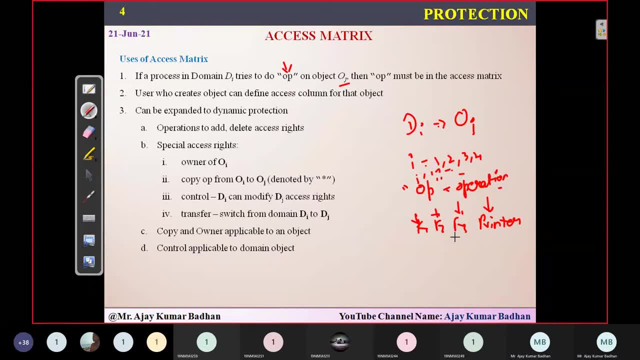 we have represented here. okay, these are the matrices, what we have exactly represented in this particular thing. so, how many objects? we have four objects, so, object one, object two, object three, object four. and this is what, for similarity, i'm representing, as oj. okay, so that is what he's doing. 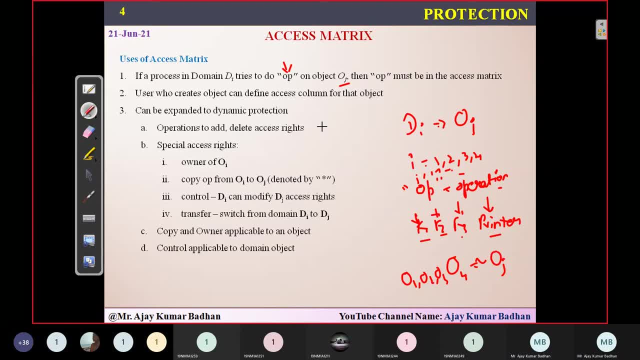 so whenever we want to create an object here. so operation, what are the different operations we can perform? here is nothing but uh, read operation, write operation and execute operation. these are the different operations that a particular process can perform on a particular object. here now, here so when we are actually. 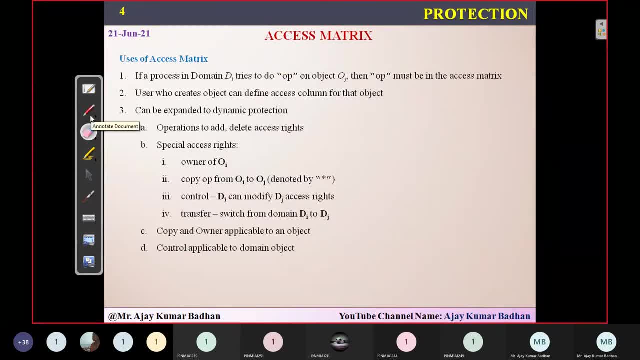 wanted to perform this particular operations on this particular access matrix. so what he's saying is there are three different type of operations. there are three different type of operations which we need to see, which we need to consider in order to perform it, something we call it as copy, copy. 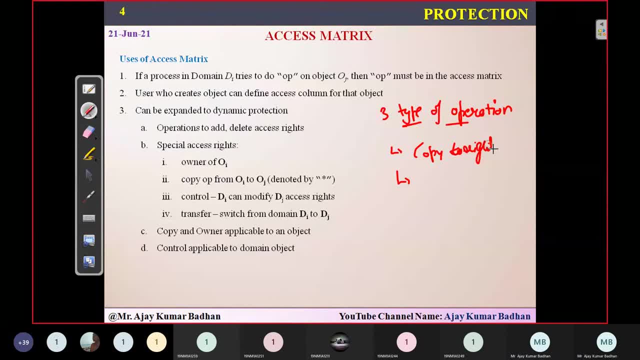 okay, so copy right, we have something called copyright owner- and then control. these are the three different operations which we need to control, or you can say that these are the three different type of space. special access rights- okay, these are already proven, presented here. this is one. so, in order to perform, and means for a particular process to execute under different, different 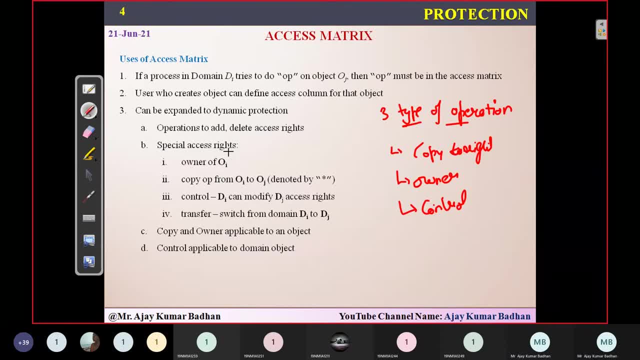 processes, or i mean on different, different objects, in particular domains, they have to have these special access rights. that is nothing but owner right, copyright control right. okay, transfer. transfer is nothing but switching this. i will explain it. this will be coming in the copy itself. when you're talking about copy here, there are two different domains. you're going to get that. 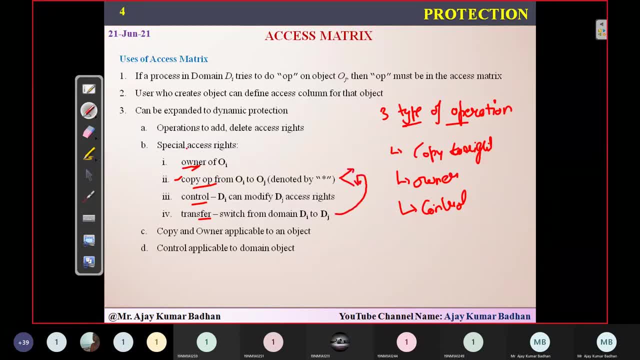 will be talking about here. one of them is transfer here, another one is directly moving from one to another copy. another one is copy. there are two different things that we have in this particular thing, and then we have something control and then copy an owner applicable to an object- control- 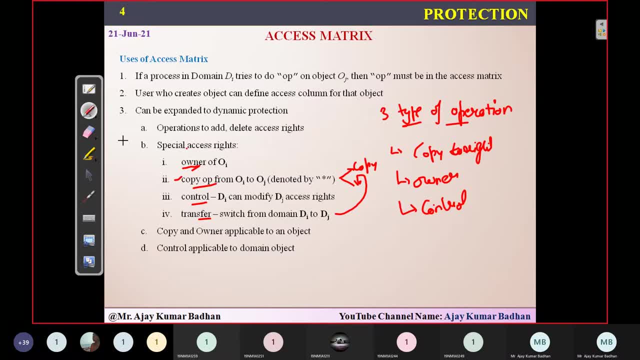 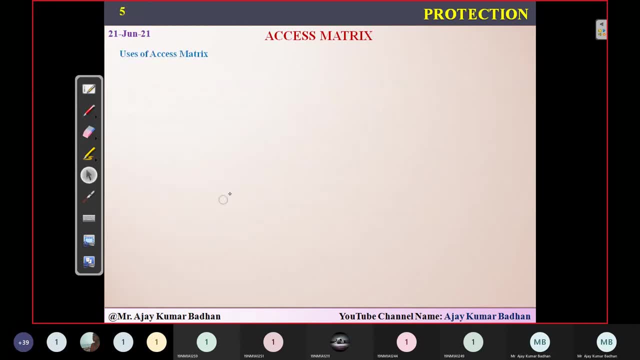 applicable to a domain objects. okay, so the i'll explain them one by one using a diagram, so that you people can easily understand how exactly this particular thing is working. let's go ahead. so here what he means to say that, since we are applying a mechanism, so this access right, this access matrix, whatever we are actually. 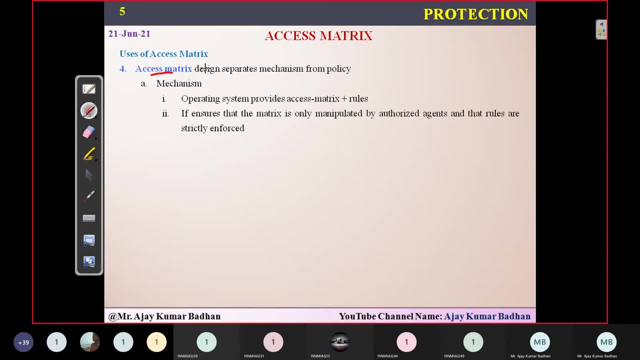 represented here in a format of a matrix. this matrix is able to provide or provide a mechanism in order to create different, different policies. we can create different, different policies here. we can create a different, different policies based upon the mechanism, whatever we are using. so what is the mechanism i'm using right now here is nothing but access matrix. so using this access, 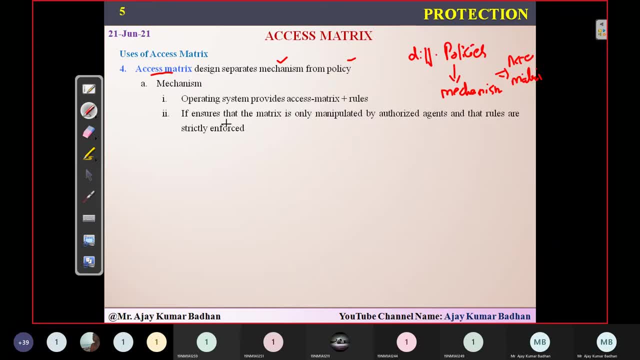 matrix. i can provide a server different type of gains, so operating system provides access matrix plus rule. that comes under a mechanism. so i will be presenting an access matrix and within that i will be representing the different rules with respect to the objects. whatever we are having, it ensures that. 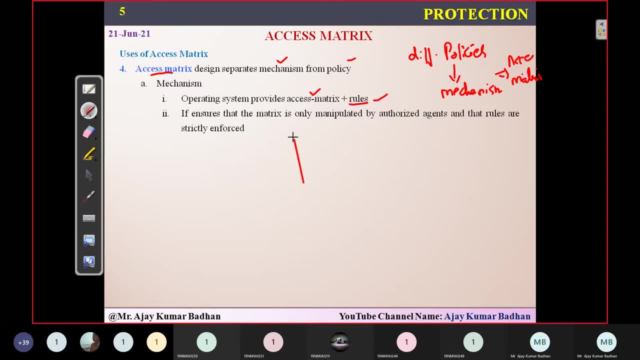 the matrix is only manually authorized agents, obviously, whoever is actually creating that particular matrix, they have the full permission to represent, like, for example, i have represented our objects here, right? uh, something like i have represented file one, file two, file three. now i have written for domain one the read operation for file one. who is actually going to decide that? 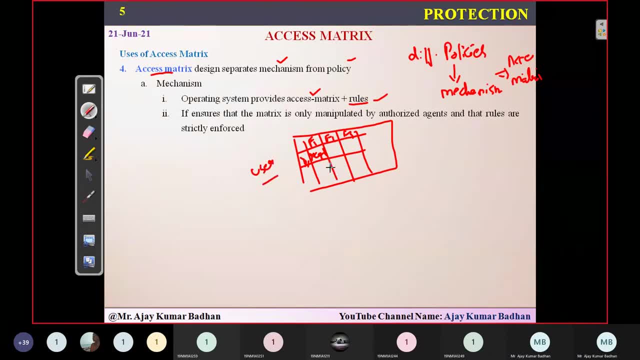 the user is actually going to decide and, based upon the requirement, based upon the environment and the requirement where we are exactly performing this, this will be decided by the user. he will be creating this access matrix and performing it. that is what he's saying exactly in this particular thing. okay, so what are the different policies? uh, user indicates. 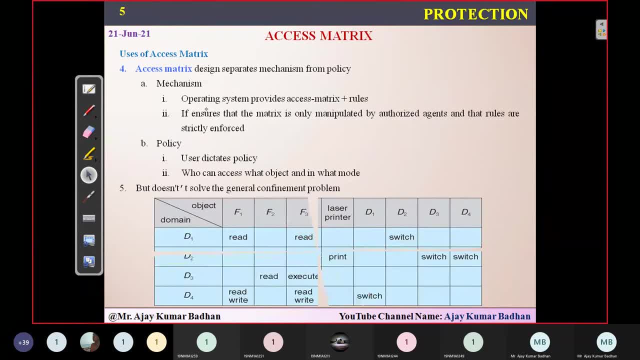 falsely so we are the one we are going to indicate, paul says here. so, apart from that, what he's saying is: uh, on the columns, what? in the columns, we were representing objects. but if you want to switch a particular process, we have already discussed in the previous session, if you don't remember. 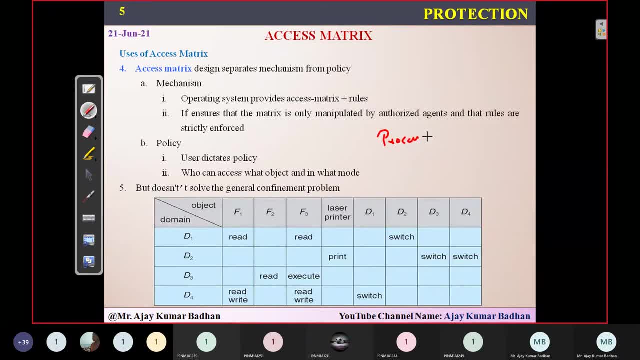 you people can just watch my video here. so in a previous session i said the process may be shifting. the process may be shifting or you can call it a switching. a process may be switching from one domain to from one domain to another. the process may be switching from one domain to another. then that case, how the access matrix is going to help. 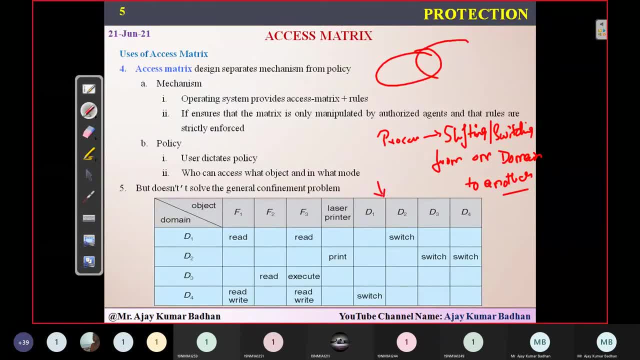 us in order to represent. you know the, for example. uh, i gave you an example like this: this is domain one and this is domain two. a process p1 is initially working on the object that is present here and suddenly this process p1 switch it to this particular d2 in order to perform some operation. 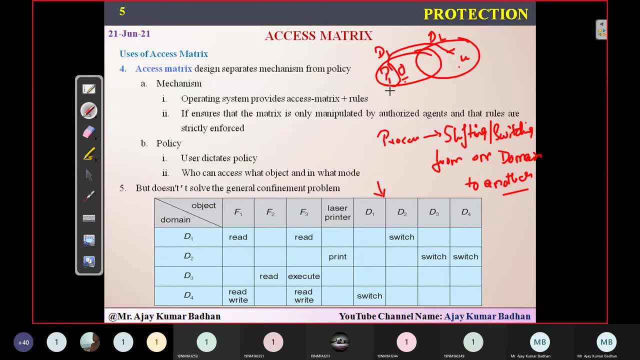 so, when this particular switching takes place by this particular process, how can we represent with the help of an access matrix? now, here the best example. what he gave is: we can do one thing: the thing is that we people can represent the domains also as objects, as you. 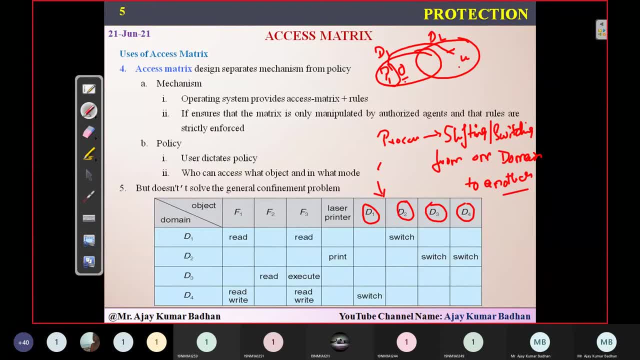 know, in the access matrix, the columns are used for representing what objects, isn't it? the columns are used for representing objects and the rows are used for representing domains. so if you see here what he's saying is, apart from the objects, whatever we are using, apart from that, we can. 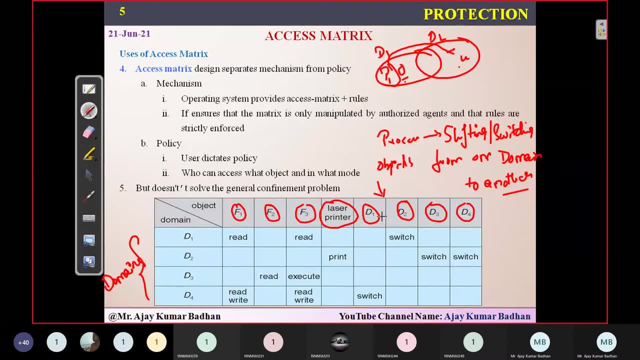 use the column matrices- i mean the columns in a access matrix- to represent the domains as an object. so here, d1, d2, d3, d4, these are the objects we are representing, and why we are representing here is that we are actually specifying some rules that not all the particular process cannot shift from. 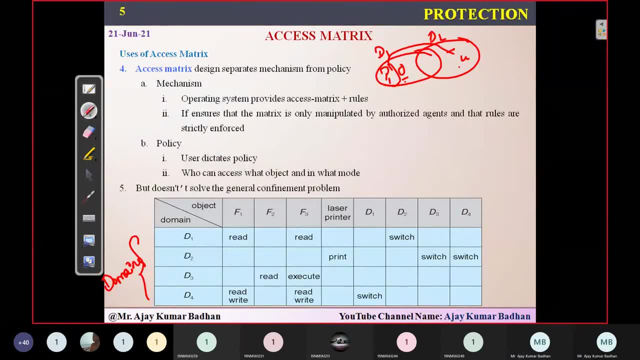 one domain to another domain easily. a particular process cannot shift from one domain to another domain as per its own requirement. it is done only based upon the rules. now, if you see here, let me explain it, if you see the first row, if you consider this particular domain, if a process is executing, 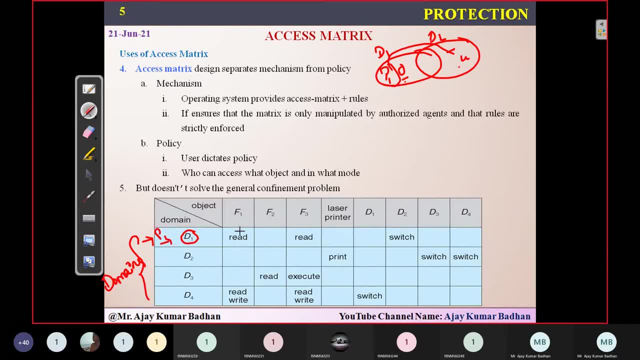 if a process p1 is executing in a domain d1, it can only access two different files here, f1 and f3. that is what we have discussed in the previous session, in the previous slide, where it can perform only one operation. what is that read operation on these particular files? 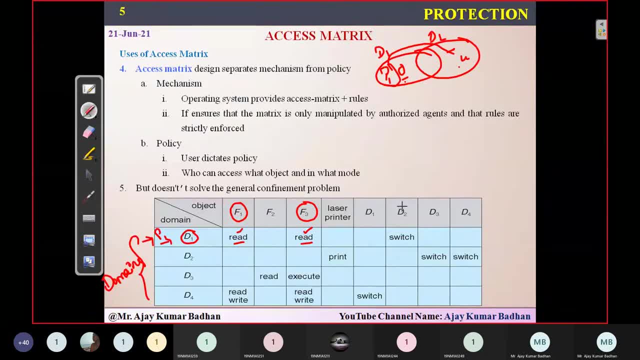 apart from that, a particular process can switch to a second domain from d1. another process means of that particular process. whichever is executing that particular process can jump from a domain 1 to domain 2.. so wherever is written, only through that particular domain we can jump. we cannot jump to some other particular. 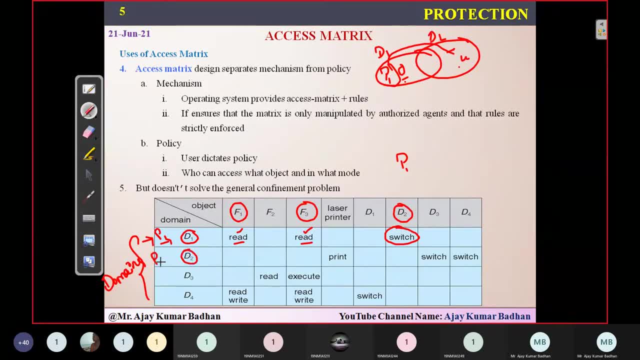 domain. for example, if you take a domain to suppose here another, suppose here another process is working. let us suppose pj. pj is that process which is executing in this particular domain, then what is the object it can access in order to perform operation? that is nothing but the object. 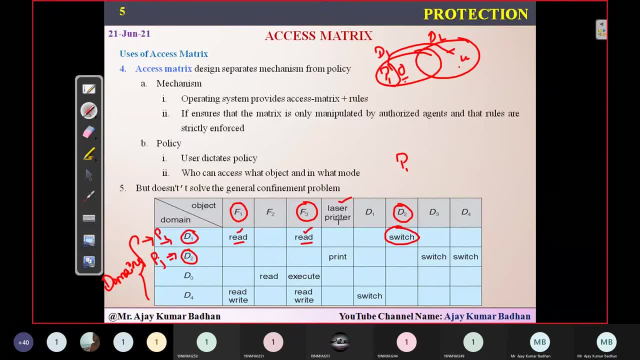 is laser printer. it can only use laser printer to perform the operation. and what is the operation? what is the operation he is going to perform here? he can only print is the one which is going to perform on this particular laser printer. now, in case this particular process wanted to jump from one location to another location, how can he jump? means: 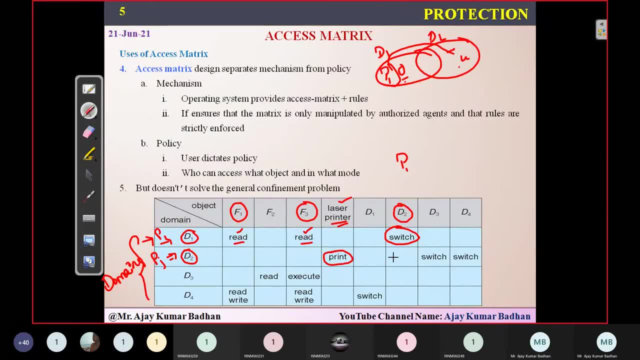 if you see here, this particular process which is executing in domain 2 can jump to domain 3 or domain pro. that is nothing but this one and this location. but if you see here, what about this domain one? it cannot jump to that particular location. so when it is jumping to domain 3, it can. 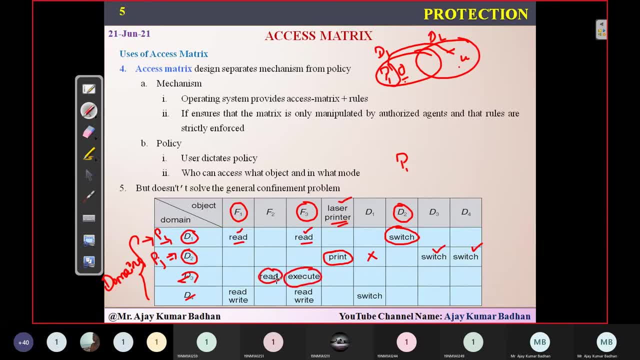 only jump to domain 2 and file 3 also, and when it is accessing them, whatever the operation we have specified here, that operation will be performed on those particular files, whichever has been specified. okay. so this is the way how we people can say: if you, if you take the last one, domain 4, if a process, 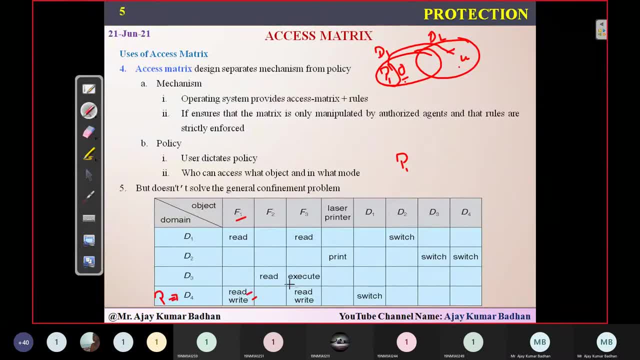 is executing in this particular domain. it can perform read and write operation on file 1, read and flight operation on 5- 3.. apart from that, if you wanted to switch to some other domain, it can only switch to domain number one. this domain, that particular process, particular process can jump. and when did it jump into that? 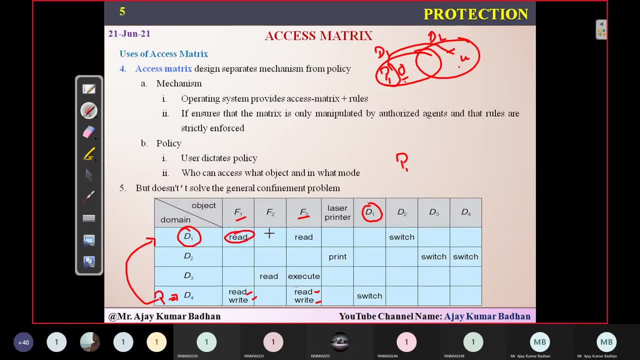 particular process. then it can access file 1 for only reading operation and file 3 for read. then it cannot perform right operation here when it is jumper to domain number one. but if you see here coming to domain 2, domain 3 and domain 4, they cannot perform any operations into this particular. 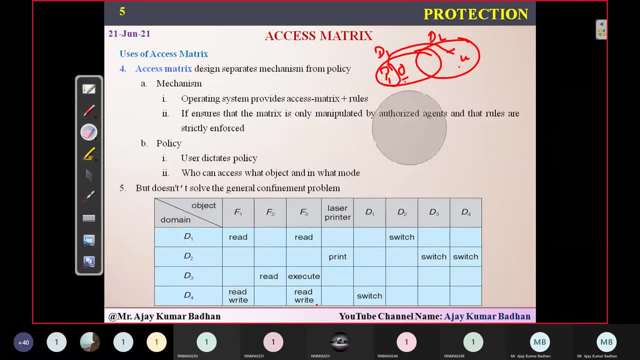 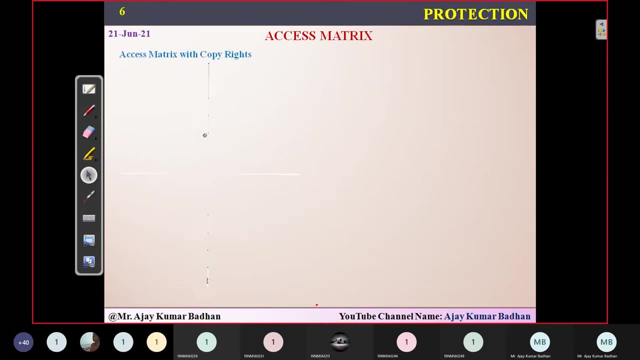 thing. this is what he is exactly saying in this particular scenario. okay, so this is the way how we people can represent switching of a process from domain to another domain. so whenever a process is jumping from one location to another location, we can perform this. now, apart from this, as i told you that we have something called as copyrights, right? 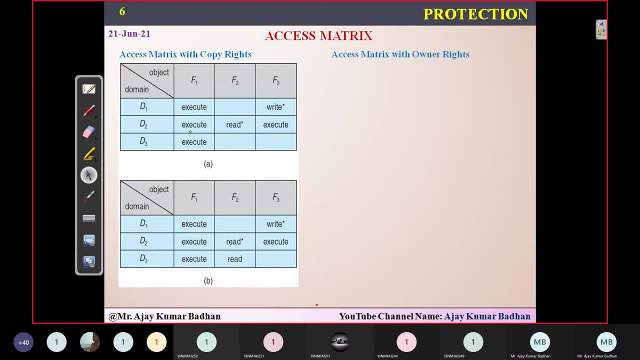 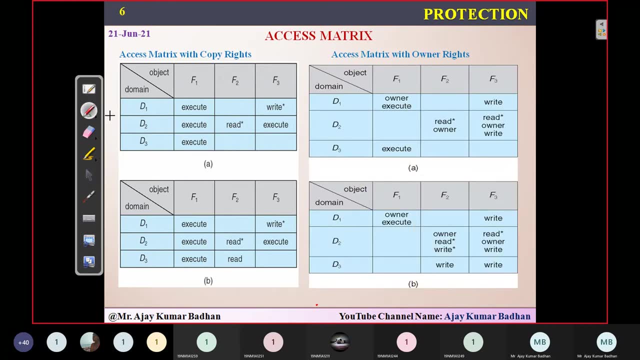 so this is a diagrammatic representation of a copyright and this is a diagrammatic representation of a owner right now. what is the difference? please let me allow you to explain this particular concept. if you see here domains, so here i am having three different domains i am representing 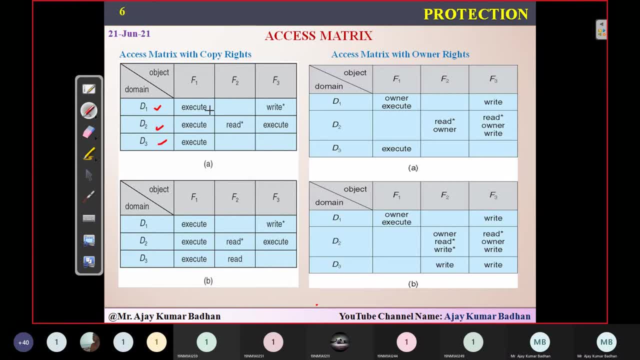 and there are three different files: f1, f2, f3, okay, and in this f1, uh, it will be performing operation, something called as execute- here execute in file one, and same way for file two or in the domain two. it can perform read operation and write execute here. so what do you mean by copyright? here is 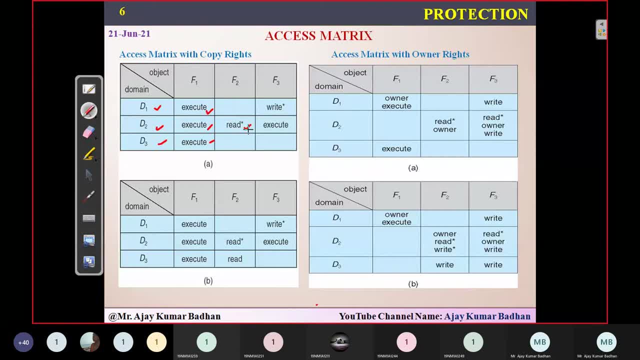 nothing but one of the operation, which is we are performing on that, that will be represented with the star. you can see, here there is a star to this particular thing, and same way there is a star right for right operation in the domain, one for the file three. we are having star. so what do you mean by star? here is nothing but. 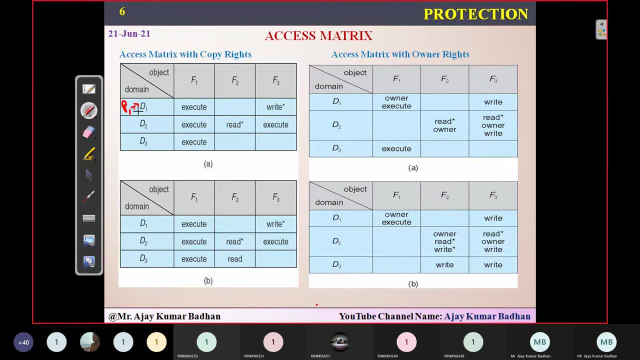 whenever a particular process. suppose, let us suppose there is a process p1 which is executing in this particular domain d1, okay, and then it is having an access to which particular objects here- file 1 and file 3- and what are the operations that can perform on those particular files? 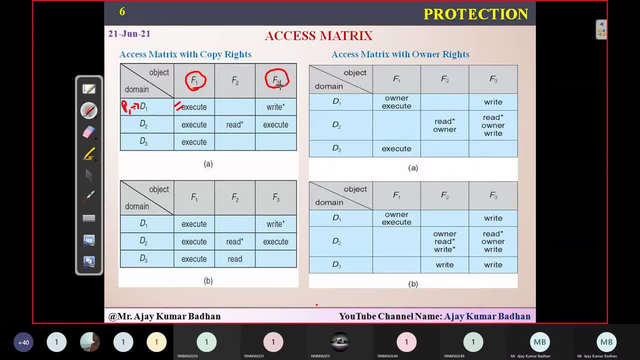 execute form f1, file 1, and write operation on file 3.. that is okay. now, what do you mean by copy? in this case is nothing but the file 3. file 3 is the part of the file 3 which is perfectly praying for. 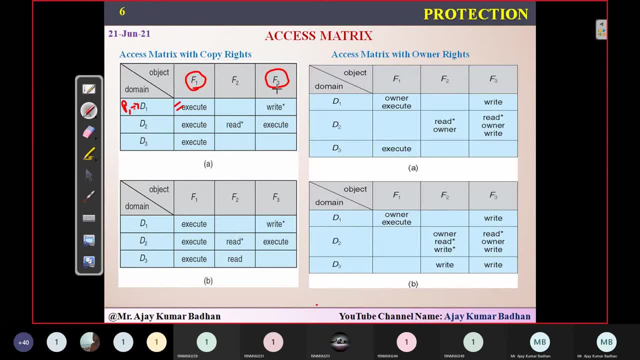 but whenever a process is executing on a particular file- I mean F3, it is having a file permission for write. Now, copyright is nothing but that particular process has a permission to make this particular write of that particular file to write anywhere else. 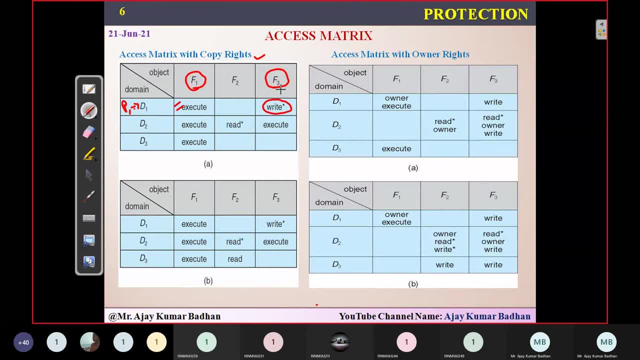 Copyright is nothing but that particular file F3.. Whatever the file we are executing, suppose the process P1 is actually accessing a file F3, and it is performing something called as write operation. When it is performing a write operation here, this particular process has a permission. 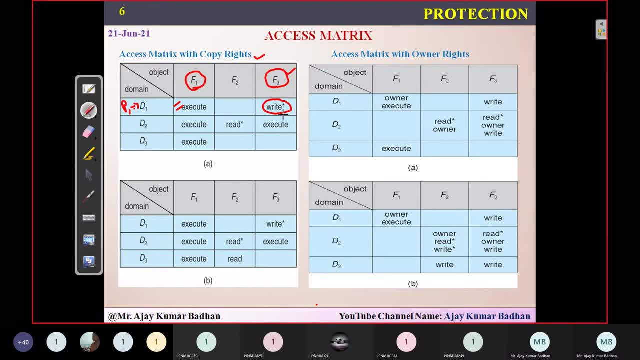 one-time permission, not multiple times, only one-time permission that it can for this particular file. it can write in that particular column anyway. it can simply copy that particular operation. For example, I have an empty slot here. I can write here, write. 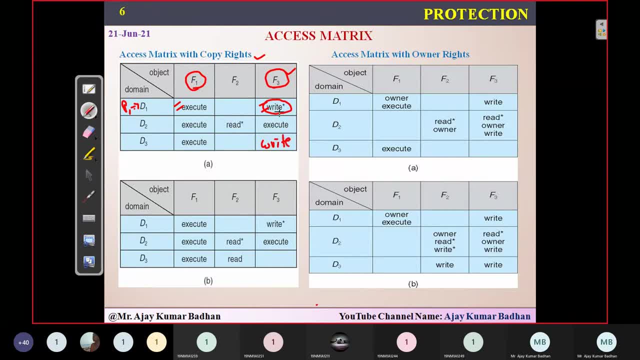 Who can write here That particular process? P1 can write here. As I said it, this is nothing but a copy of this particular file here and only one-time we can write here, not multiple times, If suppose there is no boxes present. 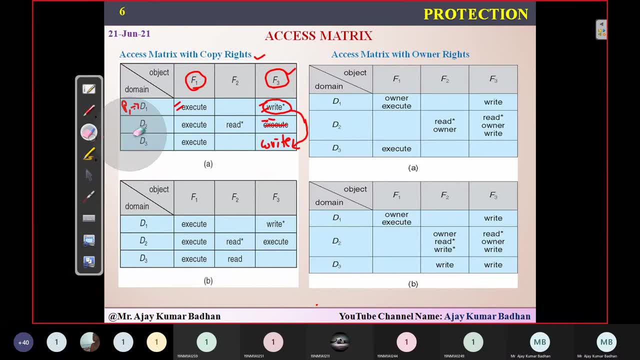 that doesn't mean that you can write also here. No, it is not possible. It is not possible. It can be performed only one-time. So that is what I'm showing in the B part, If you see here, see the domain 2,. 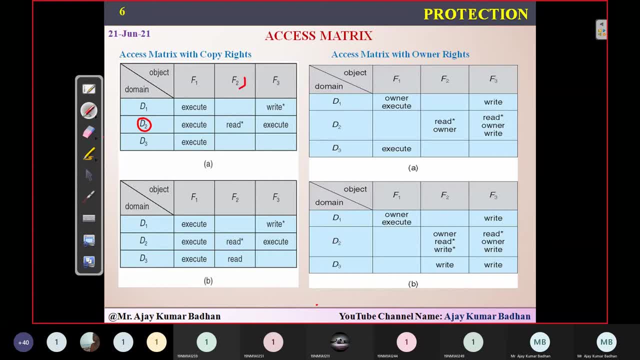 suppose the process is executing in this particular domain and it is accessing file 2, it has a read permission. Did you see that Read start Means that particular process is executing file 2 and is performing read operation. It has the flexibility that this particular read operation can be. 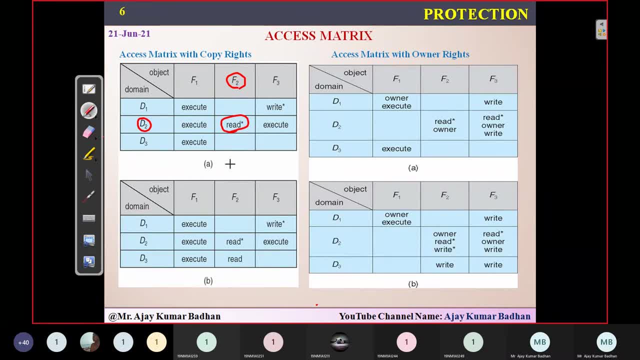 copied in any of the cells which are present above or bottom. So you can see in the B part he has copied that particular file, that read operation. He has copied that read operation for the file number 2 in that particular column in the second time. 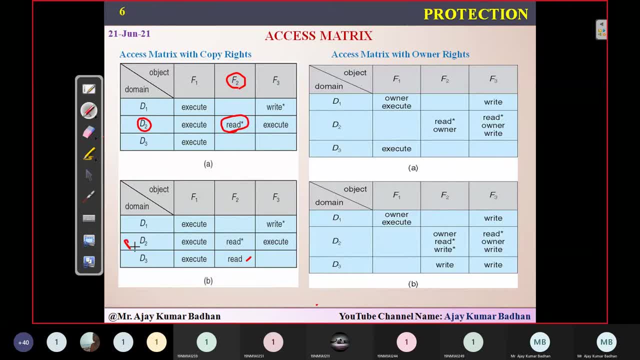 It can be done only one time. You cannot do second or third time. Suppose we have process P2 is coming, it will perform. It will perform the read operation P2 is coming. he is having the flexibility, the ability that he can refer. 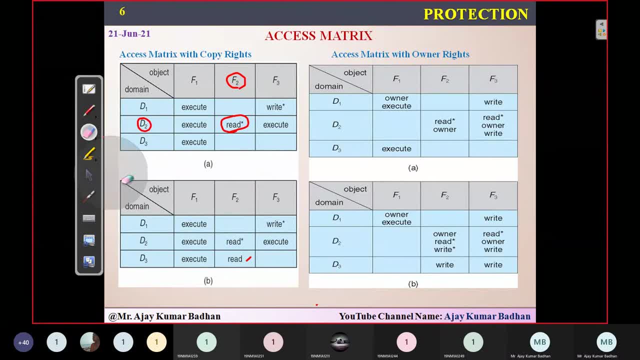 Suppose P3 is coming, Every process will have one permission to copy that particular function or copy that particular not function. you can say operation. So only one operation at a time can be accessed by a particular process and it can copy only one time. 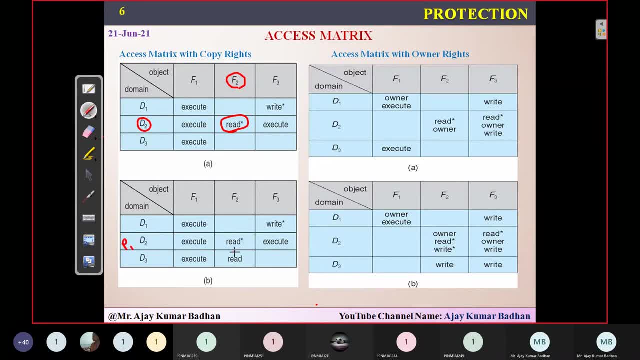 Suppose a P1 is again coming back here. First time he came here and he has created a copy. Second time he's coming again. After some time his P1 is again coming for execution. Now that doesn't mean that it can again start right here. read operation: 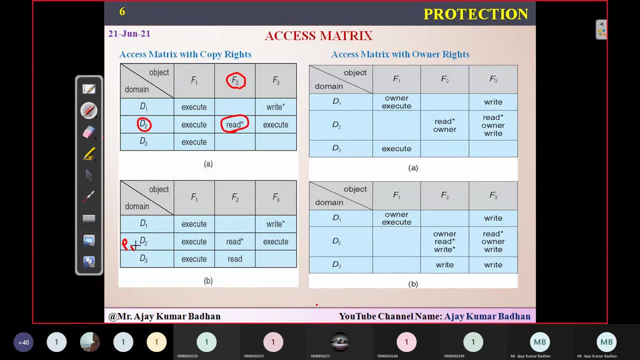 No, it cannot do that. It has given one permission to copy it. he completed, But P2 has the permission. Suppose P2 is executing it and he did not utilize this particular copyright. This particular copyright, he did not utilize it. 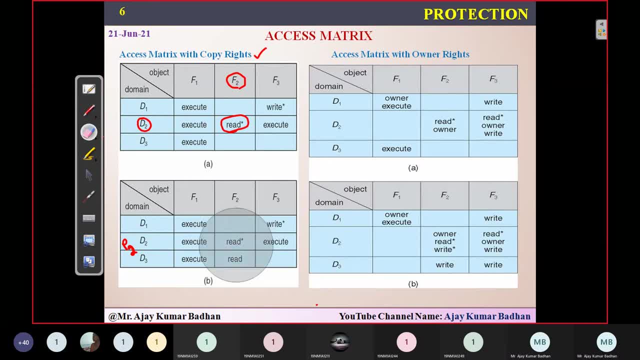 Then he can use that copyright and he can write: read X performance. this So we can copy whatever the operation we have within respect to that particular file, Whatever the operation we can perform on that respective file, wherever star is there, only that operation we can copy. 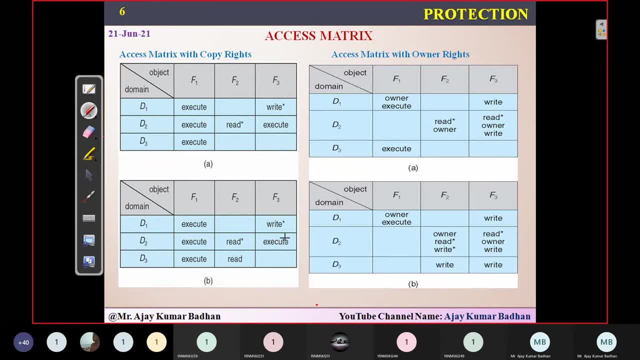 Remaining operations we cannot copy. For example, if you see, in domain two I have an execute operation on file three. So if a process is executing execute operation on file three, that doesn't mean that it can copy that nine. No, it's not possible because there is no star representation. 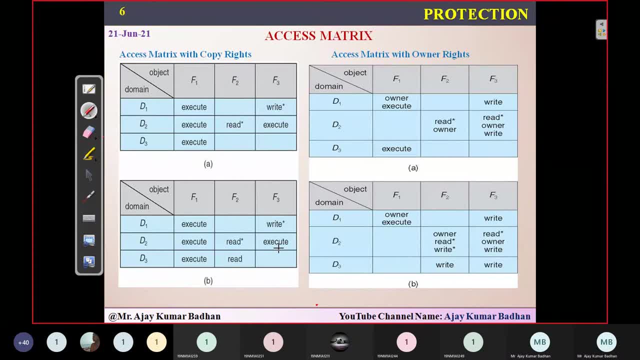 Wherever star is represented, only that particular operation can be copied. Another one. what we have here is nothing but access matrix with owner rights. Why owner rights are required here is nothing, but this is with respect to something called as domains. This is not with respect to objects here. 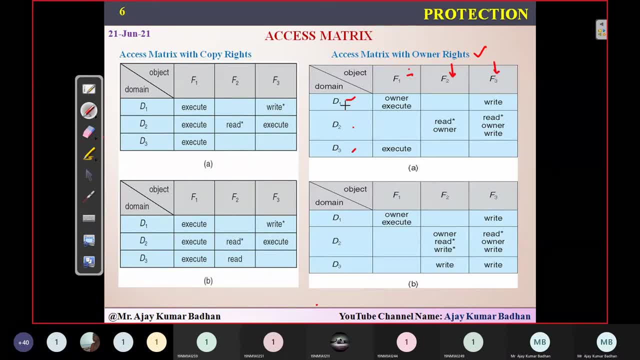 This is with respect to domain. Every domain will be a owner to one of the file. Okay, Owner right is nothing, but so we had discussed about copyrights, Now we are discussing about owner right. What do you mean by owner right? here is nothing, but every domain which we are having here. 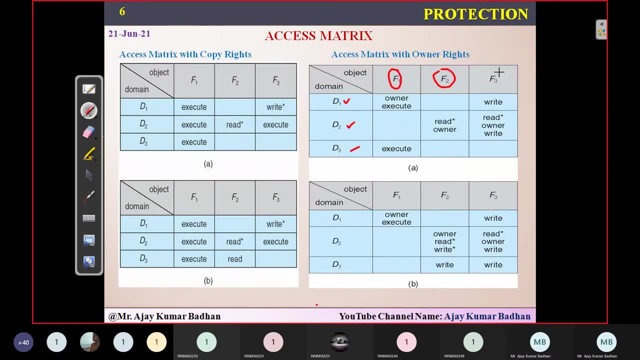 Every domain will be owner of one of the object that is present here. How many objects? we have here? Three objects: F1, F2, F3.. Among these three, one of the object will be. this particular domain will be the owner. 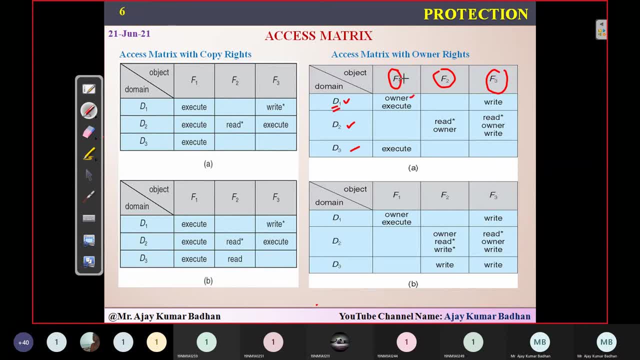 If you see here, this domain will be the owner. If you see here, this domain will be the owner. If you see here, this domain will be the owner. D1 is the owner of this particular file, but he's the owner for what? If you see here, this domain will be the owner of this particular file, but he's the owner for what? If you see here, this domain will be the owner of this particular file, but he's the owner for what? For execution purpose only. 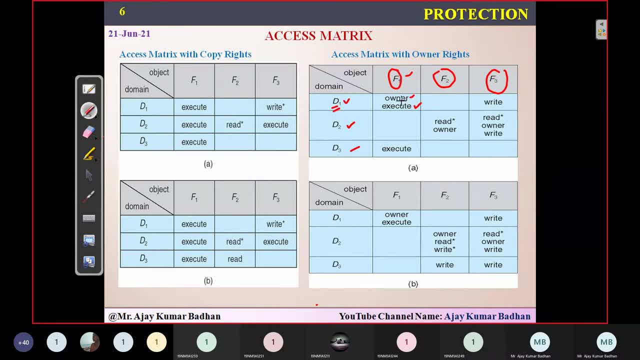 If you see here, this domain will be the owner of this particular file. but he's the owner for what? For execution purpose only. D1 is the domain which is the owner for executing file one. For execution purpose only. D1 is the domain which is the owner for executing file one. 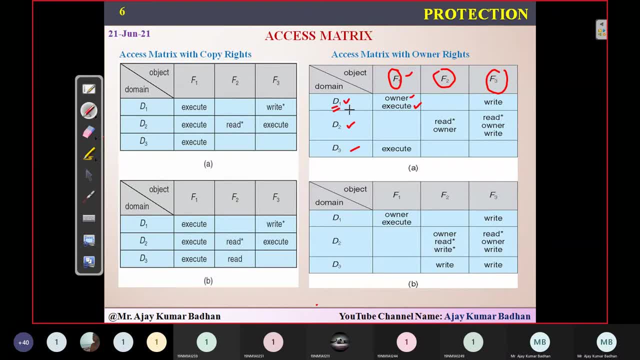 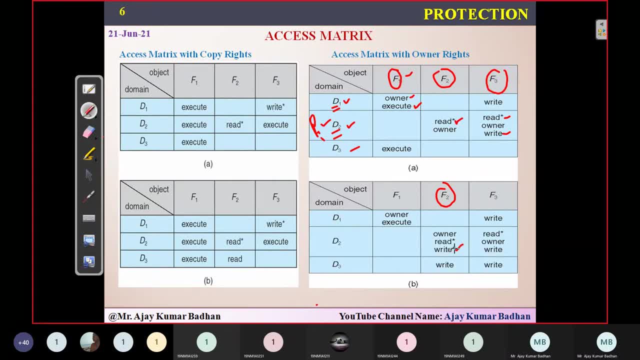 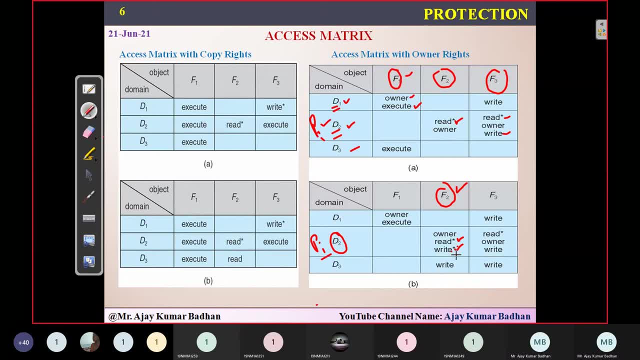 copied. suppose some process is executing. he has actually copied the right operation and he placed it. here means in the domain 3 also. we can perform a right operation on this particular f2, but we cannot again copy that to this particular location. same thing is this here also. you can see, here we 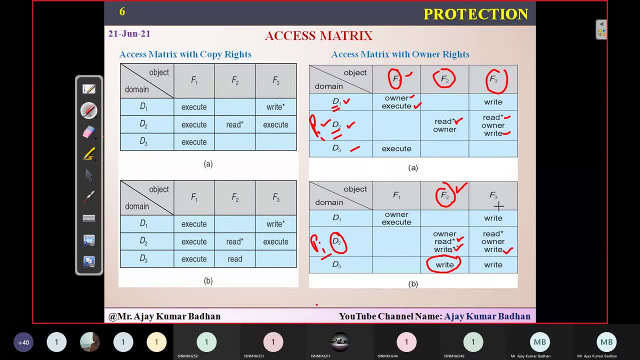 have the owner right operation, so the domain 2, what he did? is he actually within that? this? this he is the owner of this particular file. so in all the columns he has represented right operation, you can see this one. he has represented here something called as a file operation in this. 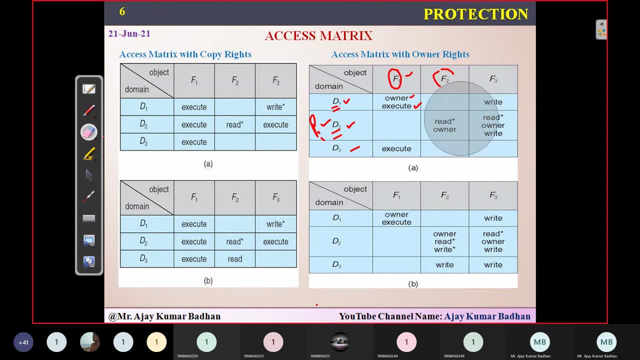 particular. yes, okay, so this is a way how exactly the owners are going to take place of. one is with respect to copyrights, where the copyrights are totally depends upon the objects. based on the objects, every object will have some operation and that operation will be having an asterisk. 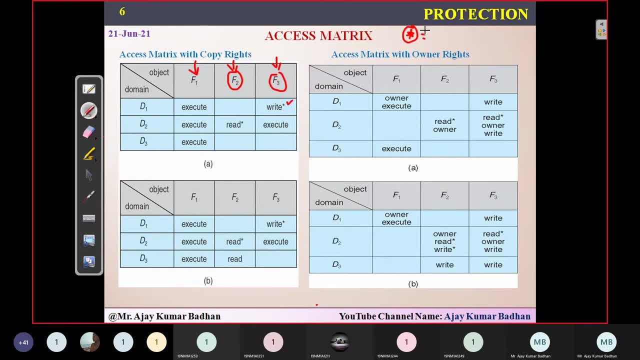 I think you people know what I mean by asterisk- is nothing but star. it means that a process which is executing on that particular file, on that particular resource or an object which is how and it is performing the operation which has been represented with asterisk, that can. 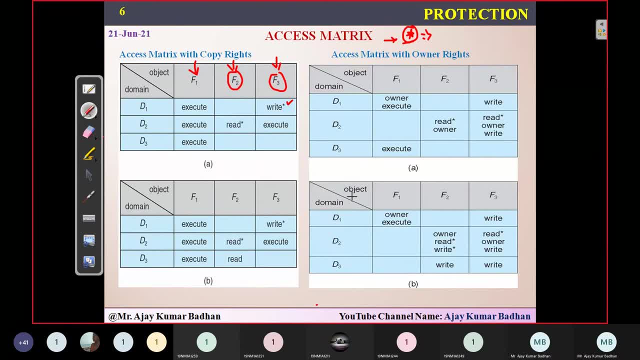 that particular operation can be copied and placed into another column sphere away, like that is what he is saying exactly in this particular scenario. when you are talking about owners, owners are with respect to domains. remember that copyrights are with respect to objects, whereas coming to owners are with respect to domain. so domains can perform the operation. so both ways he has given it, but 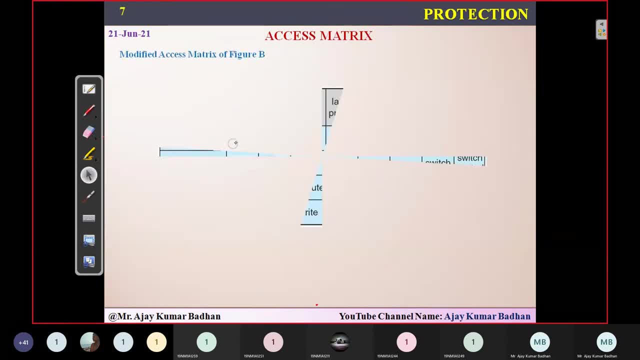 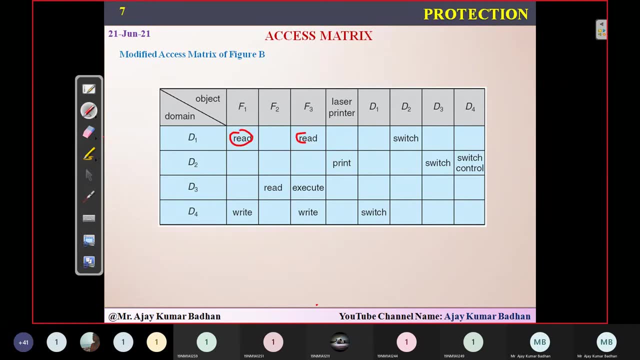 what if you want to control it, like who is exactly going to write those exactly? I mean processes and all. for example, if you see here these, read operation, read print: who is exactly going to specify? this is nothing, but the user is going to specify this particular thing. so 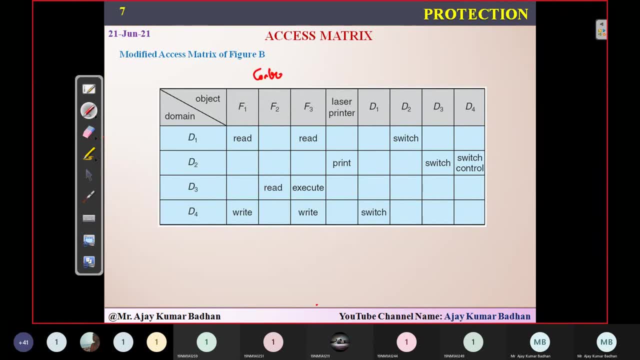 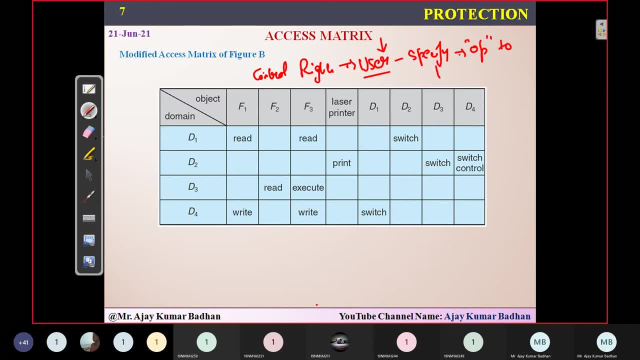 operations. so specify what type of operation to be performed. to be performed on what to be performed on different objects here. what are the objects we have on different objects? these are the objects. okay, so what are the different things we can perform on different objects? so user has been. 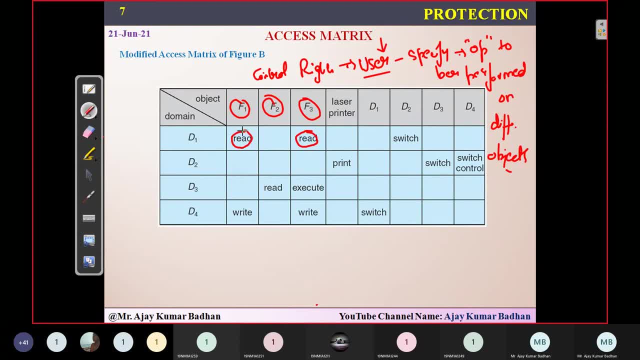 given the permission what actually operation they need to require to perform in this particular domain. in this particular domain- suppose d2 is there- it is performing print. i am as a user. i wanted to read. sorry, i wanted to write, so i will specify right operation here so that this: 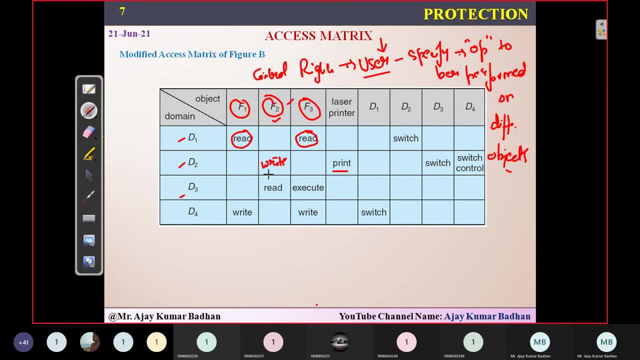 particular file. whenever a process is executing, it can perform right operation on this particular file. so i am giving the permission here and remember this access matrix. whatever you people are seeing here, this is very much important and, based on this, if a particular process is entering into this particular domain and if he is having access to this particular file, it can perform. 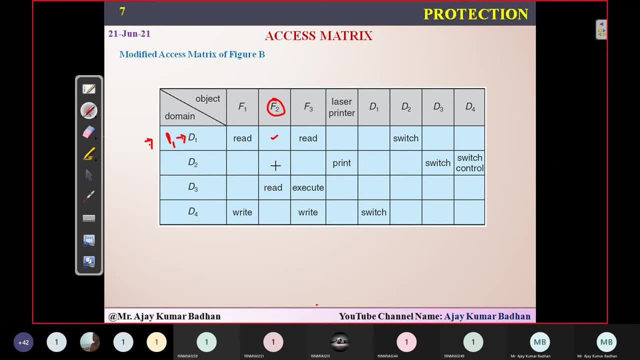 operation on this particular file only if you have specifically specified here. if you did not specify anything here, then this particular process has no access permissions or access rights to perform operation on this particular file. remember that. so if a process p1 is executing in d1, he can perform only read. operation on f1, he cannot perform. 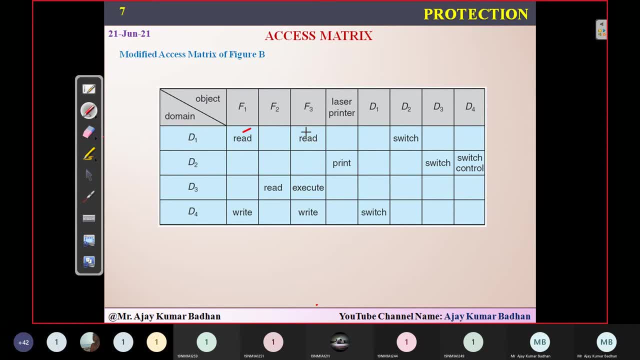 write operation or execute operation on file 1, same way for file 3 also. he cannot perform read. i mean write and execute operations on this. only read permission is allowed onto this particular thing. that is what you people have to keep in mind. please do remember that. 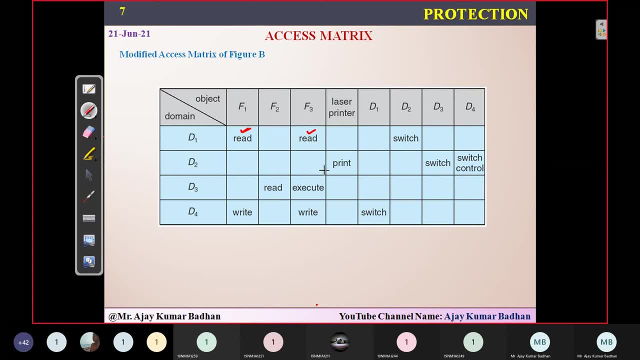 so here, what is showing is the earlier one. whatever he has shown is the control. so if you see here, uh, switching control, what we have, we can switch from one to another now. so here, access rights. when he's talking about something called as control, you can see here: 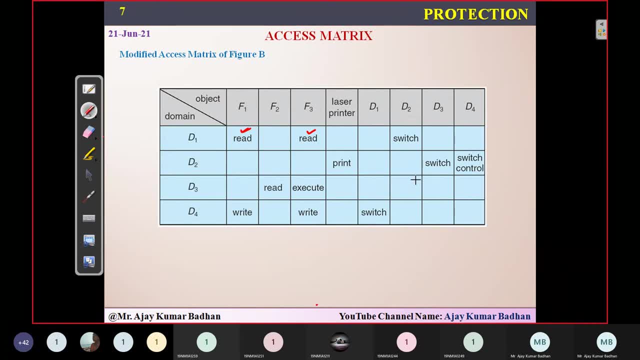 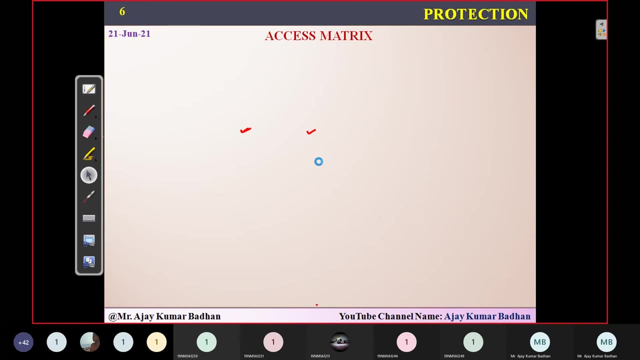 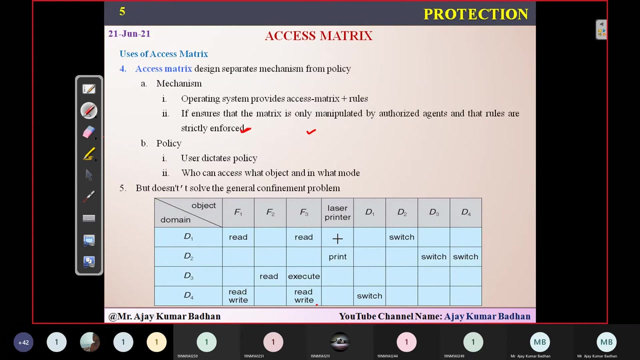 switch control, so d2, so, for example, d4, if you see the previous one. okay, let me show you the previous one once. yeah, please look at this carefully. i want you people to see the default. so when you're giving control permissions here, you people can modify the right operations here. if you see here in d4. 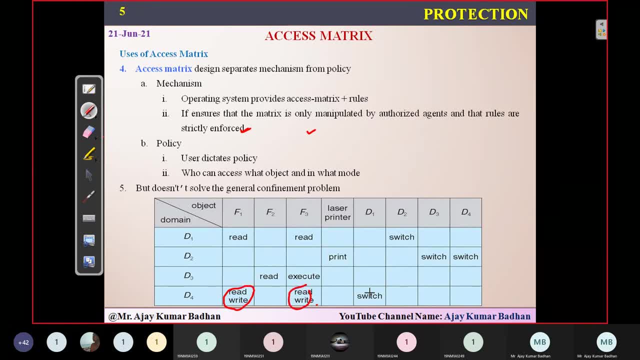 domain 4. you have read and write operation here. read and write operation here and then switch operation here right, and if you see here there is switch, switch, switch, so d. if you see here d2, d2 is having a switch operation to d4, means whichever the. 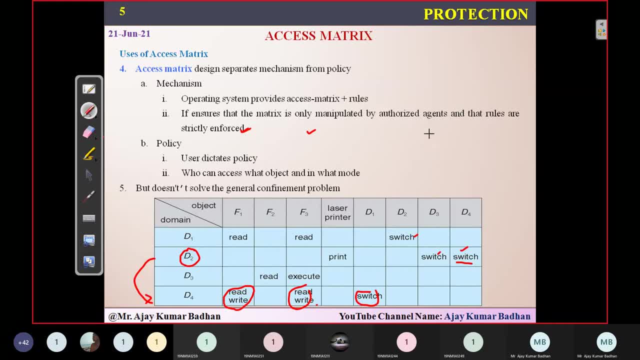 process is executing in d4, it can switch to d4. when i'm talking about control means you're giving control permission. so here i can. as a user, i can modify the operations which i need to perform on these particular objects. i can simply try to modify them. how can i? 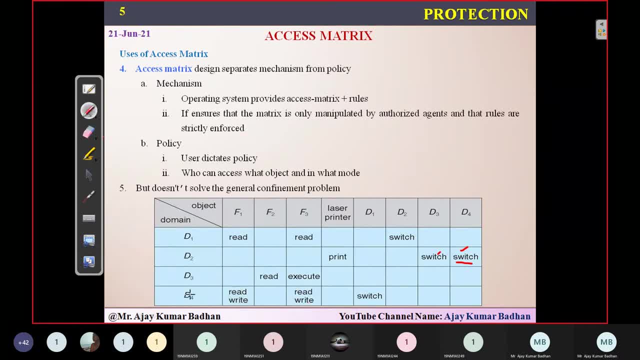 modify using control assets, so that is given to the user. so if you see here d2 is having a control switch, it can switch to d4. so here, whenever this particular performance. so here i'll give the control. i hope you people have noticed this. i have a control access, so i'm 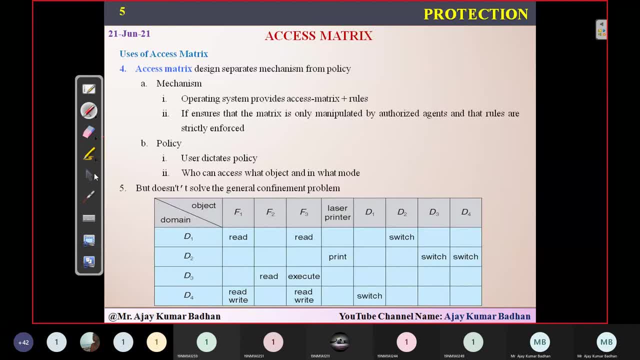 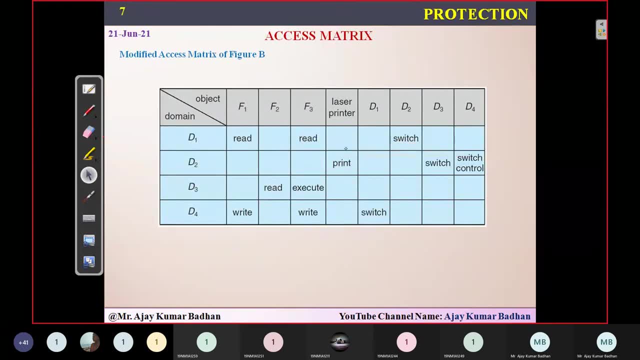 going to have something called a switch and switch, and here you have read, write, read, write and switch. so let's go to the that particular block. see here what did i do? so if you see here, there is a difference here now. so the difference here is that you are having a switch control in this particular, so not only you can switch from d2 to. 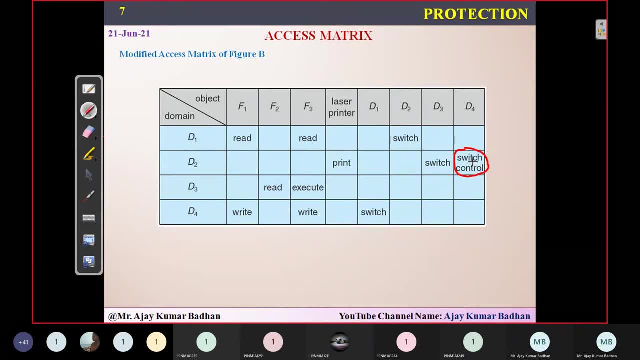 d4. it also has something called as permissions- permissions for switching the operations which can perform on this. so earlier i had here something called as read, write and read, write. but now i have been given the permission to control them, so i have removed the read operations from this particular locations. what i can perform here is nothing but only write operation. 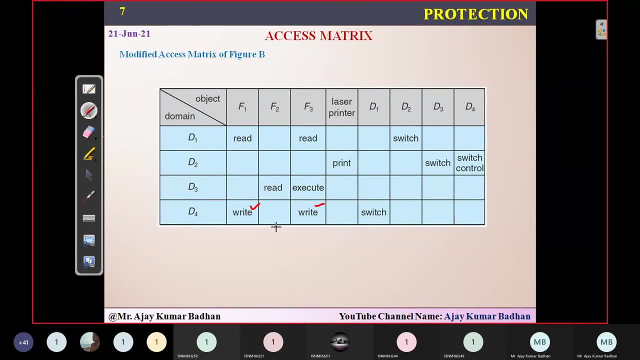 is the one which i can perform on this particular files. i cannot perform something other things, other things in the sense, nothing but, uh, what we call read operation or execute operation. earlier we are having a read operation, isn't it? so i have simply removed it. i have simply 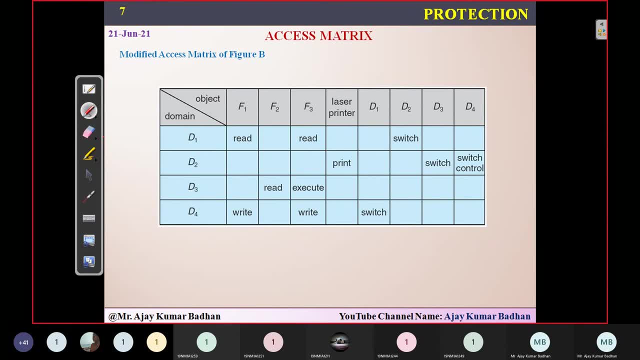 removed this particular read operations. how i am able to remove it? only with the help of a switch control. in the previous diagram you don't have control here, but now i am having a control option here in this particular case. so means i can control even the operations, whatever the operations i. 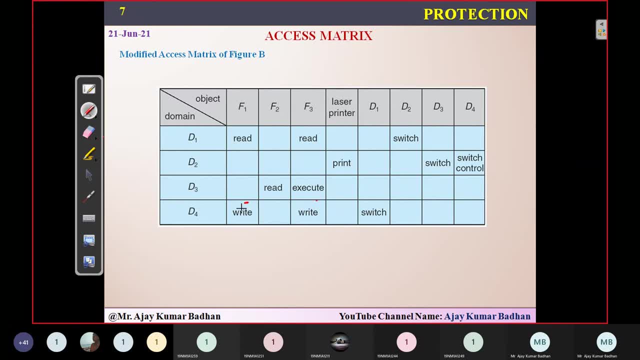 am performing here that operations. i can modify it. so i have modified. so read is there here. i removed it. here also i had a reader operation. i just removed it. so only now. whichever the process is executing in d4, it can access this particular file- f1 and f3- only for the writing purpose. it. 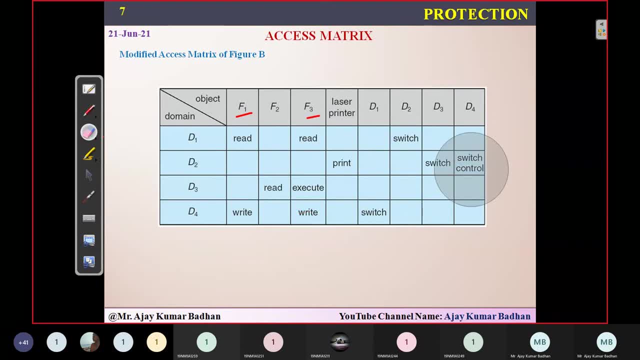 cannot perform for any other kind of things. that is what i mean to say exactly in this particular case. so let me explain all the steps to make our cross machine switch to the starting point, because this is the first step. the first step is the first step of the process of themselves. 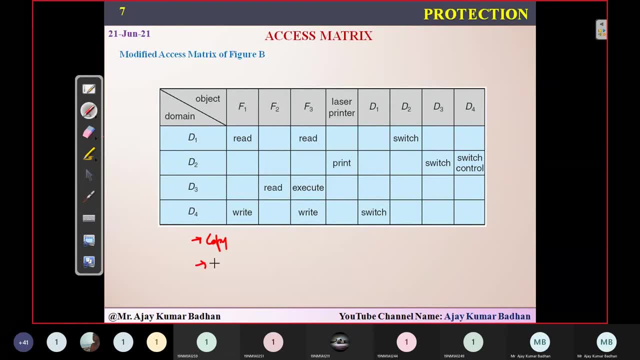 so the cross device process is the process of itself, so it is the process of the process of an operator and it is the process of all the components of an operator, and so now we are going to discuss right now how to implement them. so these are the three things that we 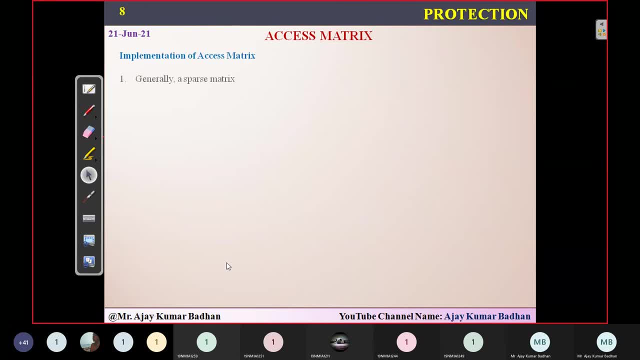 discussed here. the previous diagrams are related to copy and owner and this one is related to your control. now how to implement them. so implementation of this is actually basically the same of based upon three options. here we are having him. how can we implement this particular matrix in the program is nothing, but we can implement using some. 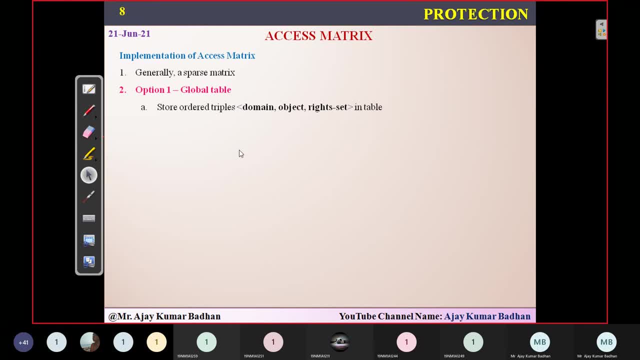 three operations. one is a global table. so global table actually consists of a paid, a pair of trip, not pair is a ordered set of triples. I can't say exactly here pain, here it is ordered set of triple because you can see, here I am having three different things here. these are important. if this pair is there, then 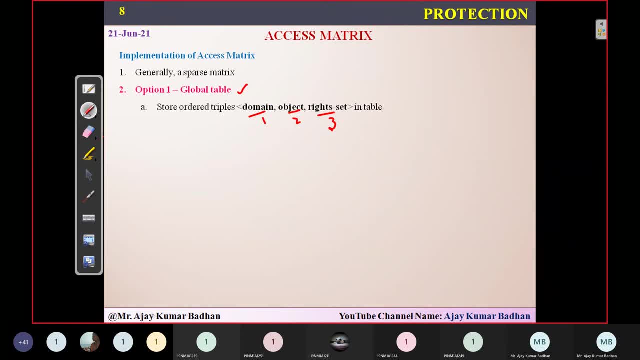 only you can implement this global table. so within the system, we will be maintaining this particular table. this table will consist of three sets. I mean is set of three different features. first one is domain. I think you understand what do you mean by domain. so the all the set of the what is the domain we? 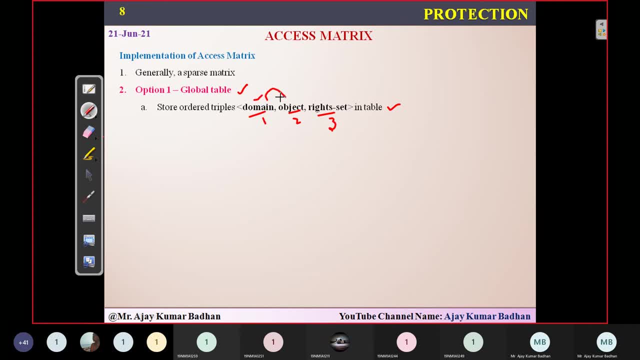 have with respect to domain. what are the different objects that this particular domain can assess that that set of objects will be represented here and on those opera objects, what are the different operations we can perform that are represented in this particular right set? okay, so this is what you have to. 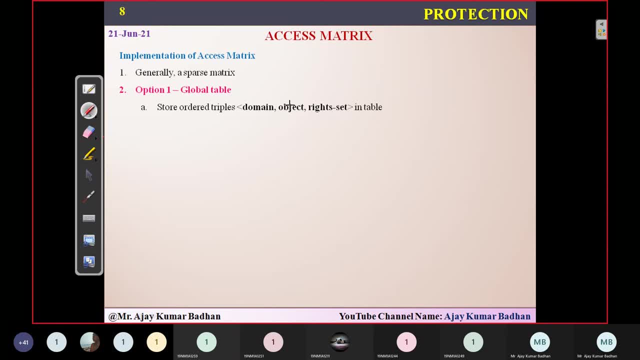 keep in mind whenever you are implementing this particular table. you have to keep in mind whenever you are implementing using global table. so this is a set. so here it is representing domain. let us suppose domain one. earlier you had a matrix domain one, and in that I can assess what are the objects, I can 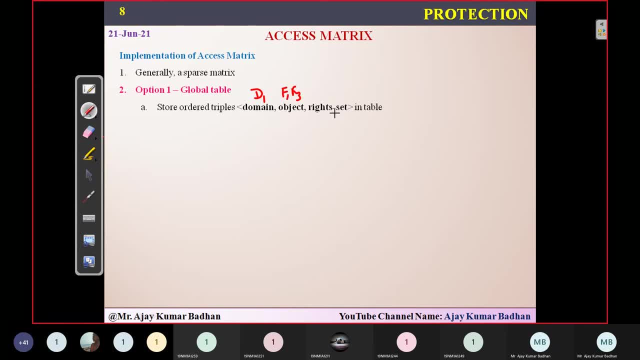 assess f1 and f3. so what are the right? I mean, what are the right operations? well, what are the different operations we can perform on this? I think I have given only read operation, so this is the one particular domain. so on a domain D1, I can assess two different files, f1 and f3, and the 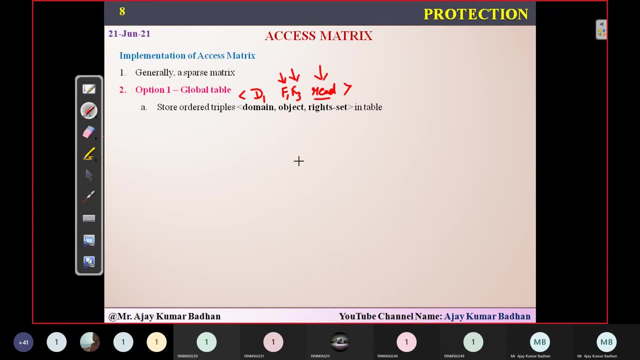 operations which I can perform on this file is nothing but read operations. okay, so this is the way how we represent it. okay, in this particular way. so whenever you people are trying to create a process and perform some operation- m suppose this is operation- you want to perform it first. what happens? the system will look into this particular global table. 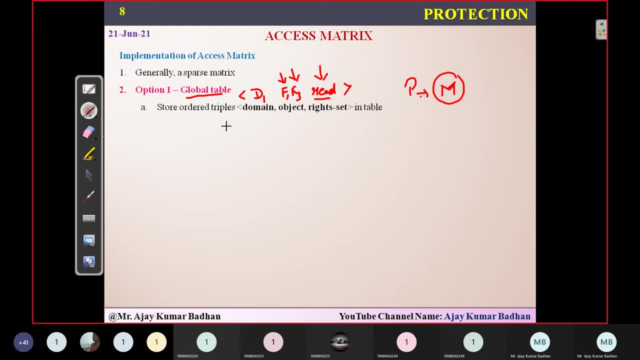 this will be maintained in our operating system. we will be maintaining this in our operating system and there we will be searching where exactly this particular global table is, and there we will try to first search this particular pair. first we will try to search this particular page and once 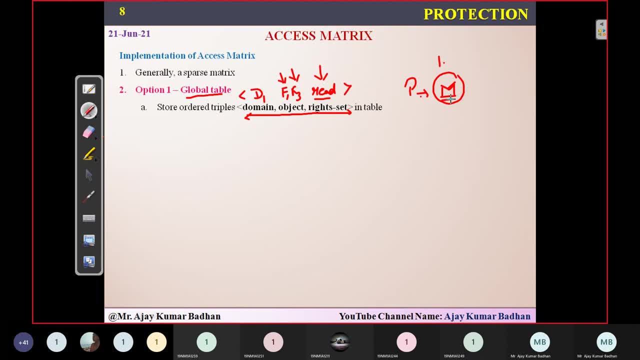 you people got this particular pair, then we will search whether this operation is present in this particular right set or not. that is what we have to see. whatever the operation you want to perform, m whether that m is present in that operation or not. or suppose you want to perform read operation. 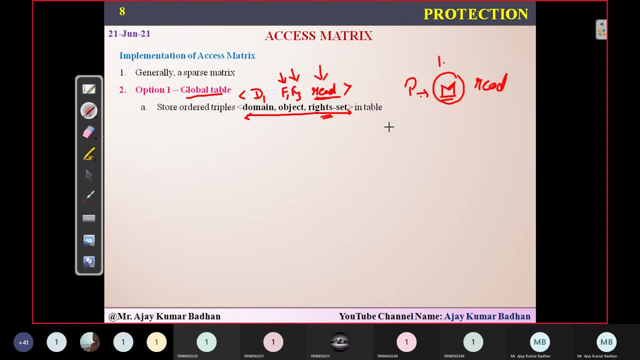 so you can see that a read operation is already present in the set, then you then that particular process can start executing read operation on that particular file. and you can see that the read operation is already present in the set, then you then that particular process can start executing read operation on that particular file. and 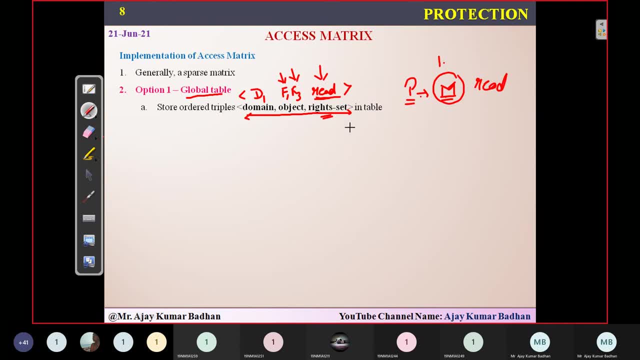 then you, then that particular process can start executing read operation on that particular file, and else it is not going to execute it. this is the way how people are providing protection, but there is a drawback here. what is the drawback here is, since you can see, there are three different things i need to store here, so definitely it requires a more memory space. 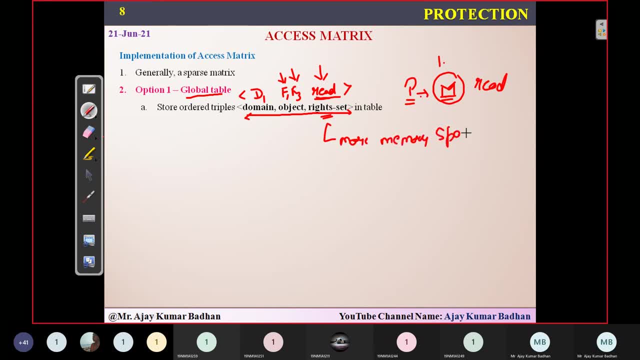 it requires a more memory space, and which is what we don't have. we are limited, so we cannot store this table, so this table cannot be stored into your main memory. we cannot store this into your main memory, so that is a drawback. so to overcome this, we have to use some special ibu. systems means additional devices we need to use. 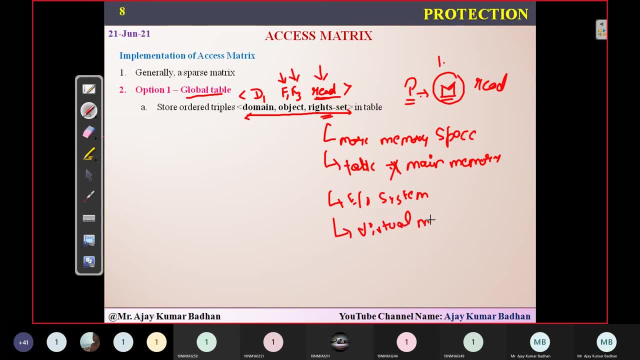 or we may be using uh virtual uh memory management, uh in order to store this table. however, it is very typical. you know it is not possible to store this in your main memory, so definitely it is somewhat typical, but still, the users are actually using them and performing the operations on this. 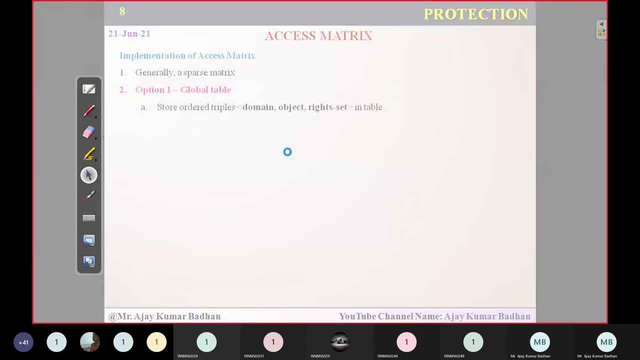 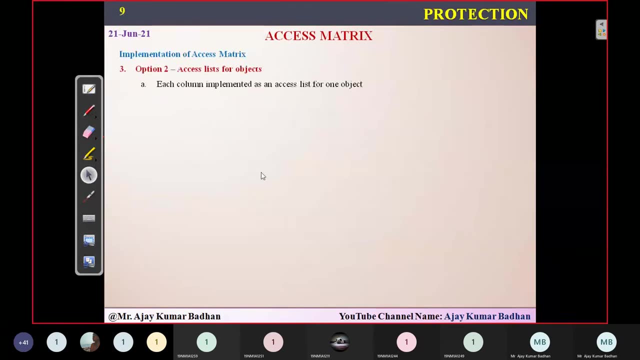 okay, so the next option: what we have here is nothing but access list of a file. so what do you remember? access list for the option is nothing, but this is a column representation, what we have. okay, so you can see here every column. so here this is nothing, but access is with respect to the 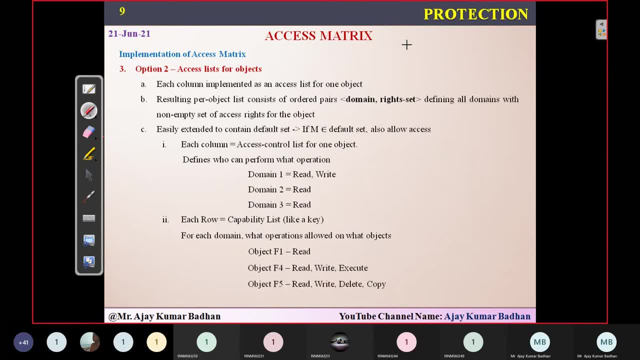 columns. what are the columns we have here? so in the columns, if you see, here in the columns we represent file 1, file 2, file 3, and then we had something called as laser, isn't it? so here, file 1, uh, access list is nothing but it is a list, it is a set of list, represent it is a pair of. 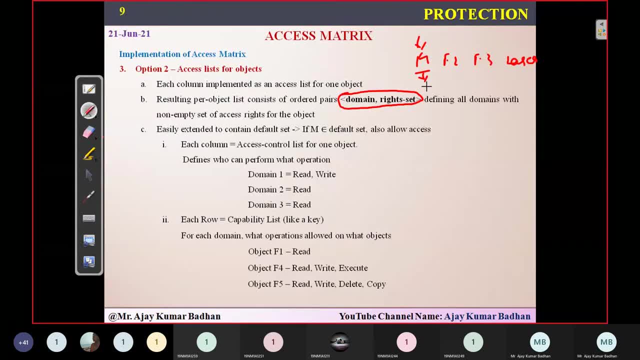 set of list represented like this, and for this particular file within that particular list, what are the different operations we can perform? that we will be representing in the right, as right sets, and the set of domains which can access this particular file, f1- that will be represented in this. 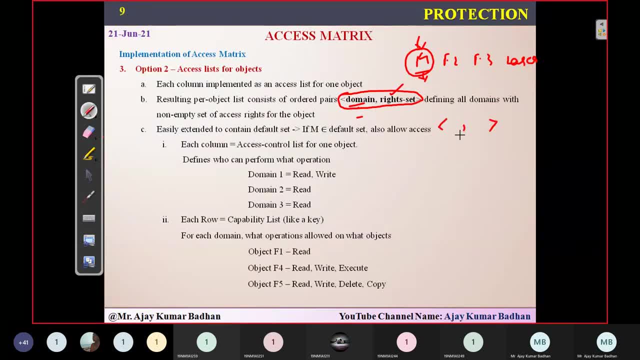 is also a pair, that is a triplet: the earlier one, this is a simply a pair. so here the set of domains, set of domains which can access these particular files that we will be representing it, and what are the different operations we can perform on that particular file that will be represented here in. 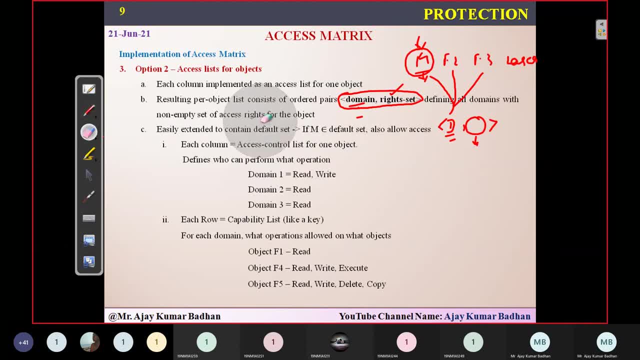 this particular thing. that's what exactly he is explaining here in this particular scenario. yeah, okay, so if you see here domain one, so if you take domain one, read and write operation can be performed on file one. so in domain two you people can perform read operation. domain three: you can perform read operation here. so this is with respect to 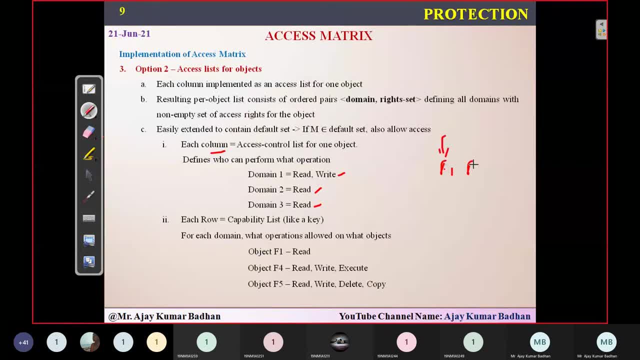 your something called as column, so column only now. so file 1, file 2, file 3, so wherever emptying- suppose here i have a read operation, this is empty. this is right operation. this is domain 1, domain 2, domain 3.. so you can see that this particular file is. what are the operations? 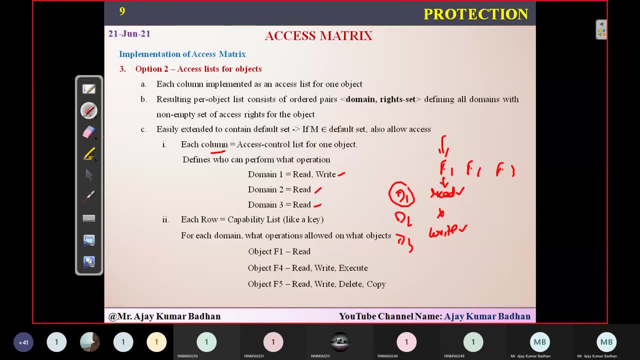 we can perform on that read and write operation, and that is with respect to domain 1 and domain 3. so that will be where i think. so d1, d3, what are the operations we can perform? read and write? this is the way how we can represent, i mean within the brackets, like this: 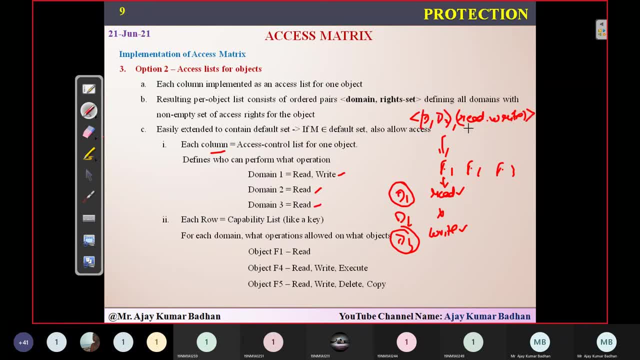 and greater symbol. this this is the way how we can represent it. so if you see domain one, read, write operation, it can put domain one only read operation. i written, so read will be performed. domain two: it is no, so it there will not be anything like this. to domain three: write. 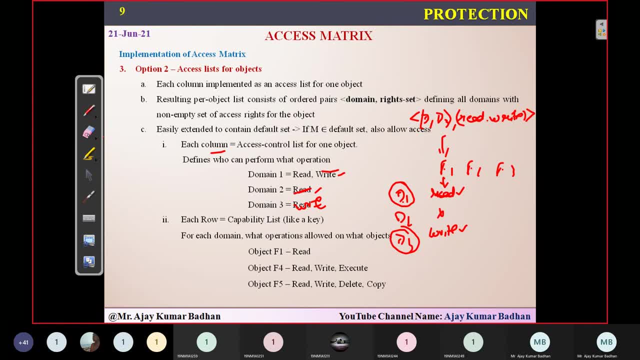 operation. so here it will be right: operation. so this is the way how we can represent. same way you can represent column wise also. so column wise is nothing but file one. you can perform read operation, read, write, execute. so whatever we have represented in the access matrix, that only. 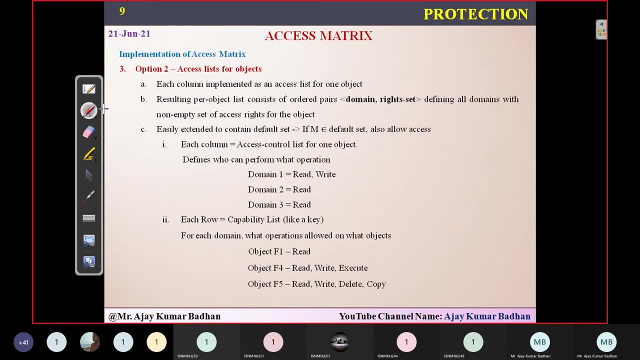 we are representing in this particular asset state. now, in this, apart from this particular pay, you are also having something called as default list. we are also having something called as default list. so whenever a particular process try to execute an operation m first, the system will try to search for this particular process and it will try to search for this. 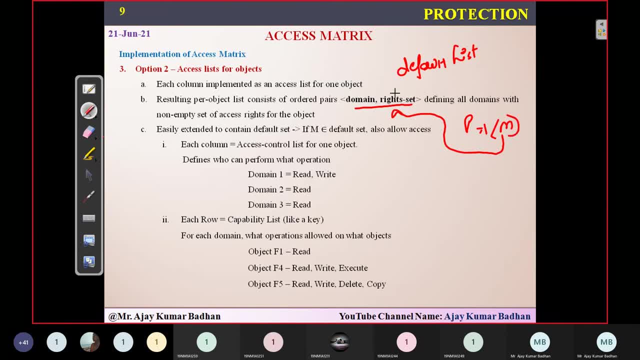 particular pay, this particular pay is available and this operation is present in the right side, it will start performing the operation. in case of that particular operation is not there there in this particular list, then it will search the default list if if in the default list you are. 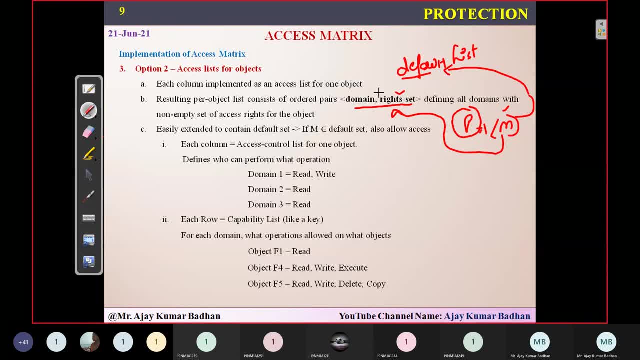 having the this particular operation, then the process can execute. but in case, if it is not present and there's an either in their default list of operations, then this particular process cannot execute this particular operation on that particular file. remember that that is that is75 condenser dom более ac importante que script zero. you cannot have this process. 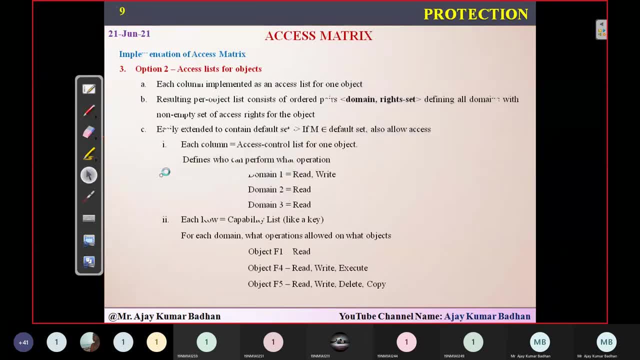 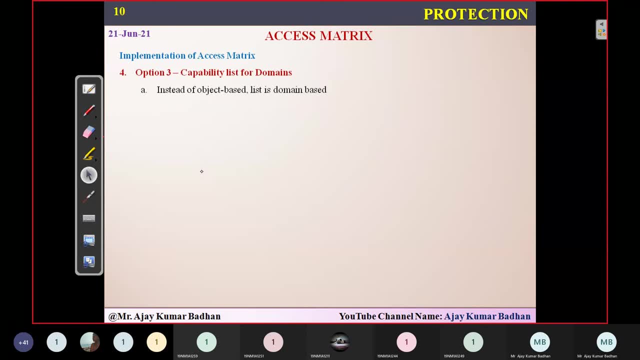 unconstructable. you cannot have this. let, as a case or any ob, remain relationshiparbeit what you people have to keep in mind at this. okay, and then coming to the third option, capability list, no, this is with respect to domain. this is with respect to domain, not with respect to your. 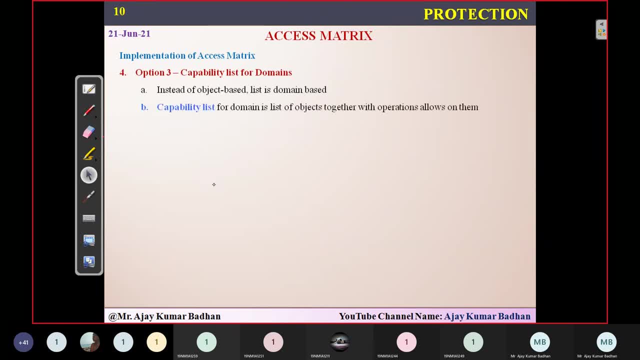 access list. i mean your files, not with respect to your objects. this is with respect to your domain. so every domain is having access to certain set of objects and they have certain operations on them. so we will be preparing a capability list. a capability list is a one uh based upon the domain. 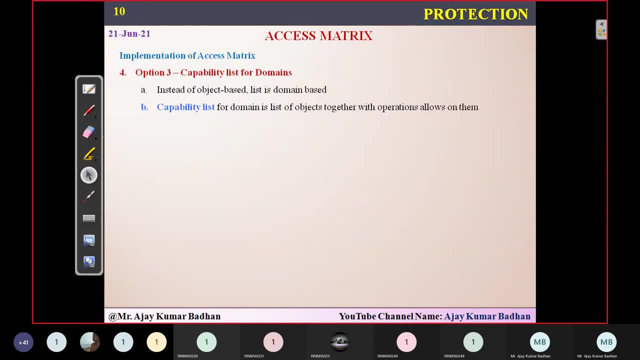 whichever the domain- that particular i mean- based upon the object, whichever is with respect to that particular domain- is available and whatever the operations we can perform on that. based on that, we'll be creating this particular capability list. so here objects can be represented either by their physical names directly or based upon their addresses, and that is what we call it as. 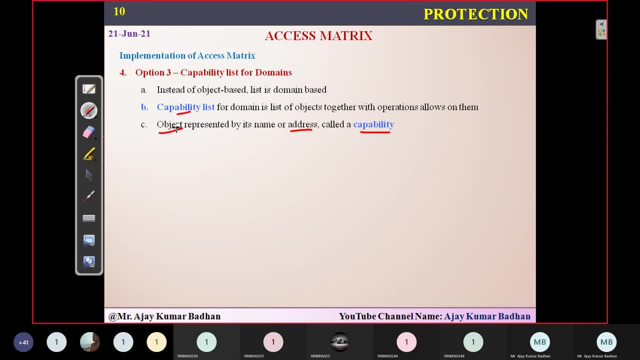 capability. remember objects. what do you mean by capability? here is nothing, but whatever the object is there within the access matrix, that is, can be represented by a physical name or it can be represented by the address. is that is what we are calling it as capability? that is what we are exactly calling it as. 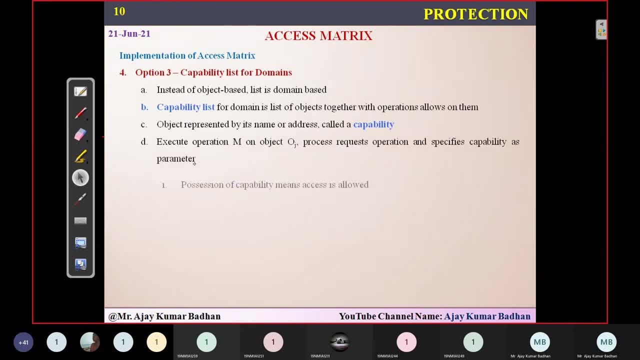 capability. so whenever an object has to be so, same thing. whatever i'm explaining from the beginning, same thing. so whenever operation m has to be executed on a particular object, first the process will be requesting that operation and specify the capability. now the system will try to detect. 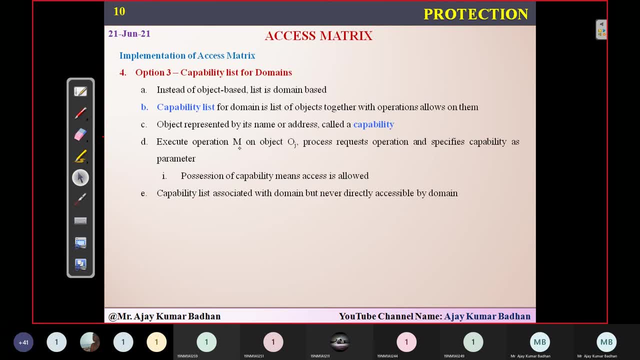 whether that particular operation, whichever that particular process want to execute, is there or not within this particular capability list. if that particular thing is not present in the capability list, then that particular process cannot execute this particular operation. but in case, if the operation is present in this capability, 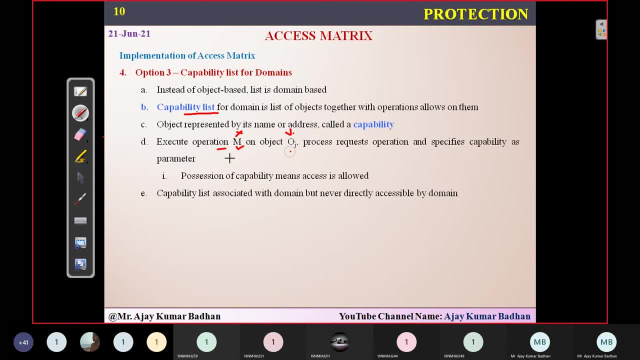 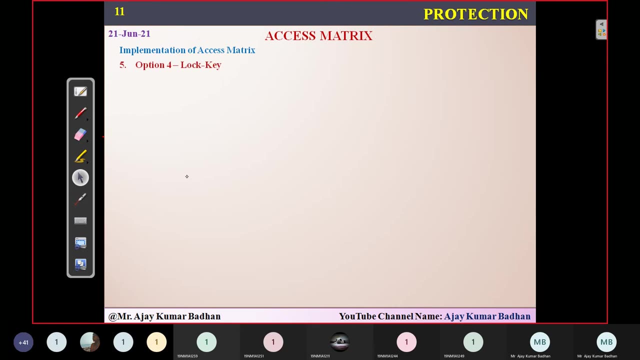 list for this object, then it can start performing that particular operation on that particular operation. so that is what comes under your capability list of domain. so here we also say something like a secure point or something like that. also, we can specify this and perform it. and the last but not the least, what we have here is something we call it as a lock key. so here we 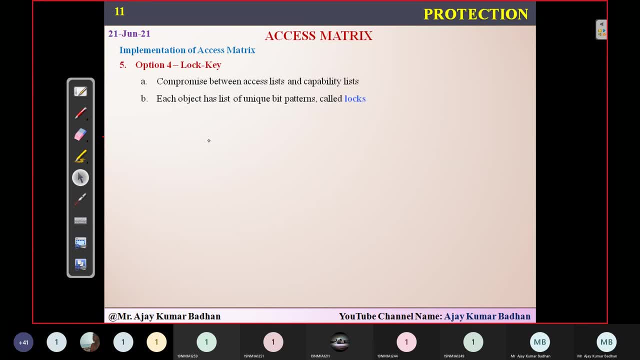 lock is nothing, but it is a compromise between access lists and capability list. access list: what do you mean by access list here? in this particular thing, access list is nothing but with respect to your objects column representation. capability list is with respect to your domain domain representation. whatever we have that, we are representing it. so every object which has a unique 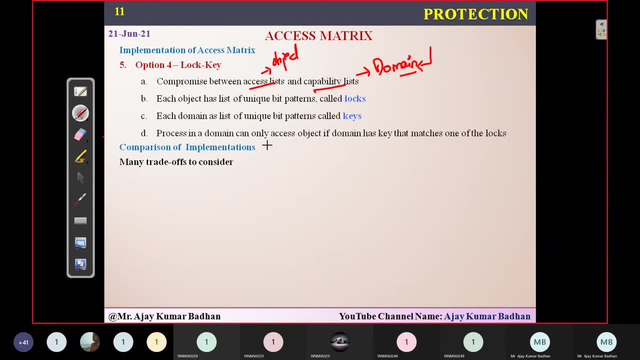 bit, every object which has a list of unique bit pattern- here we call it as a log here- and every domain. okay, so, domains we are representing now. so the domains, whichever we are representing, they will have a unique bit pattern, called as keys, and every object, indirectly. what i mean, uh, what i want to tell you in short, you people can represent that every object will. 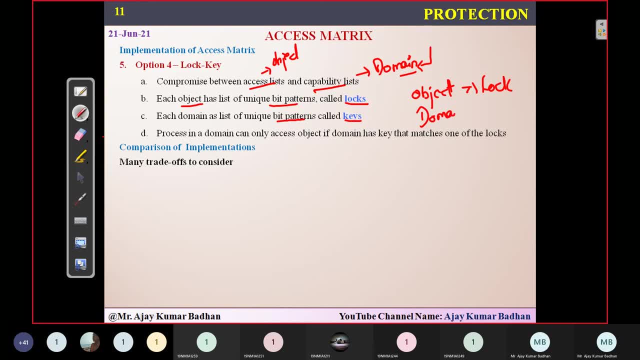 have lock and every domain will have a key. so whenever a particular process want to execute anything, this particular domain, he will have a key and he will try to search for a lock for which this particular key will work and that object. only it can perform the operation, or else it cannot. 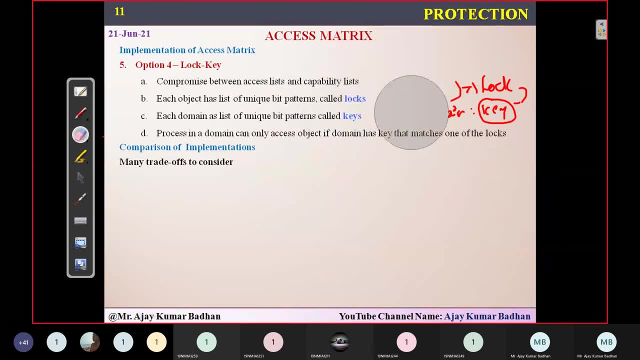 perform that particular operation. okay, so every domain will have a key with respect to the lock. so this is something like read operation: is there, so it will have. so here we'll be having a read operation with respect to this particular lock and then it will be accessing it, and then it will. 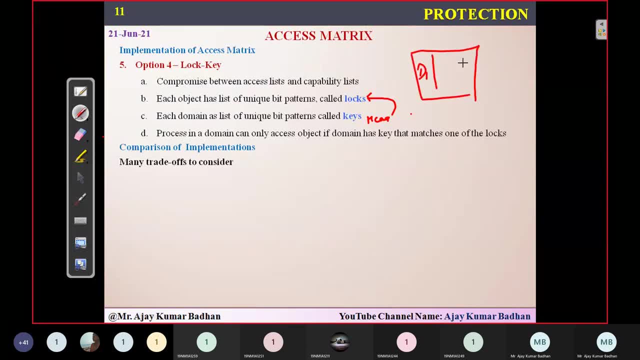 perform the operation like in the matrix. we had domain one here, right, and here we had file one. here we had read operation. now this read operation will be acting as a lock. okay, so read operation is a lock for this. and what about key here? this will be key, here is nothing, but read operation will be. 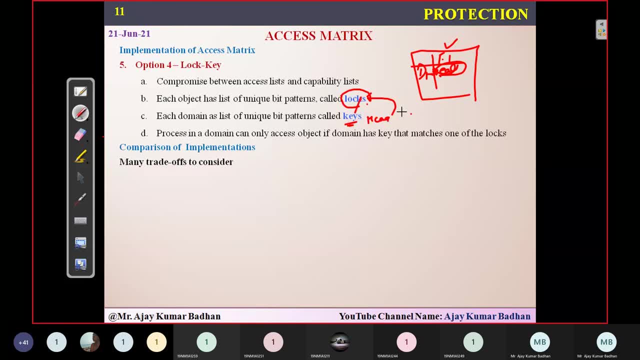 a key for this particular domain. so when this particular key and lock matches, then that particular process can perform operation on. that particular process means whatever the file or whatever the object we are having in that particular place. that is what he means to say exactly in this. that is not, that's what, nothing else. this is a normal, different kind. 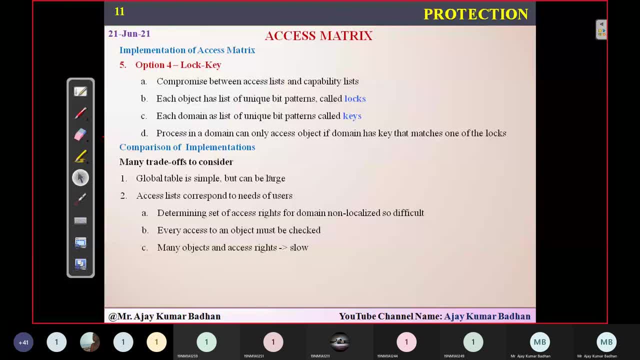 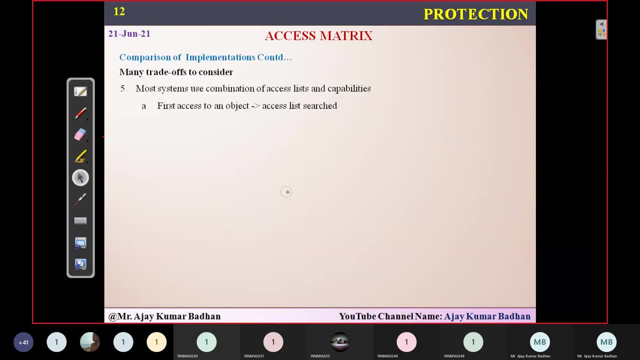 of thing. so there is a comparison here. they say that first this is better, second one is better, and later a combination of those two is much more better. this is the way they are exactly representing this, and normal trade-offs have been considered here- that by using a combination of 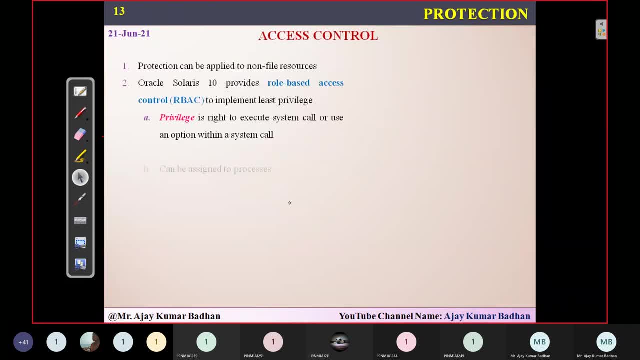 both capability model and another model, we can perform the operations well enough. so he has given certain privileges and okay. in the next session we'll be discussing about asset strikes. this is actually- this is a new topic. what we have, this is all about we have with respect to your assets matrix, and these all will be discussing in the 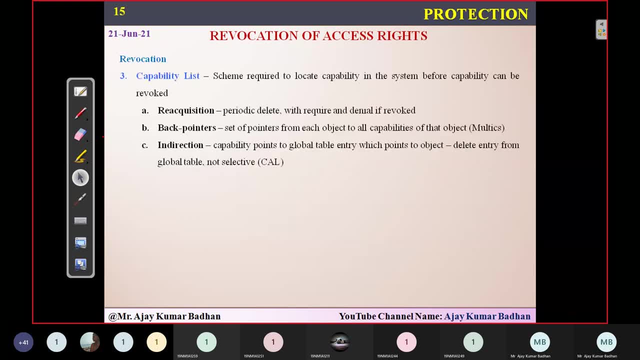 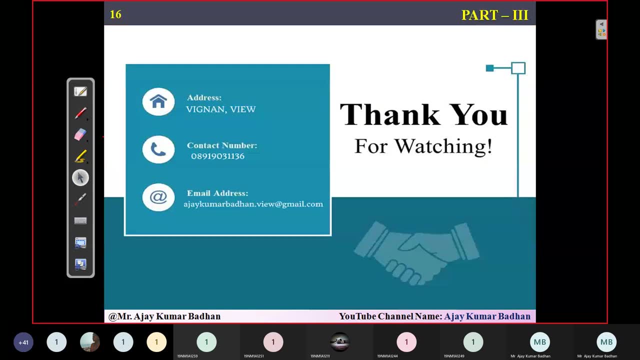 next session. okay, that is nothing but assets rights. till now, we have seen assets matrix. now how this assets matrix, whatever the assets rights we are having that will be seeing in the coming session. so i hope you people have enjoyed watching this particular video and you understood this. 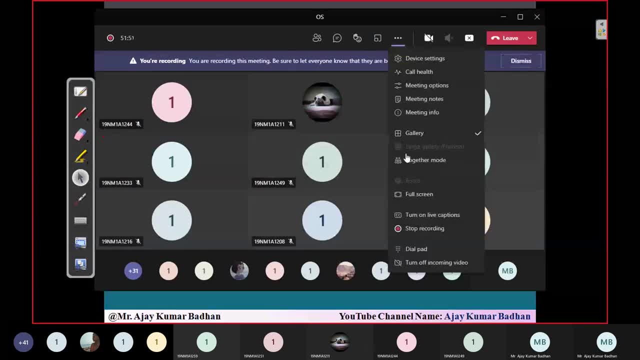 particular concept. well enough, okay, thank you. thank you for listening to me.